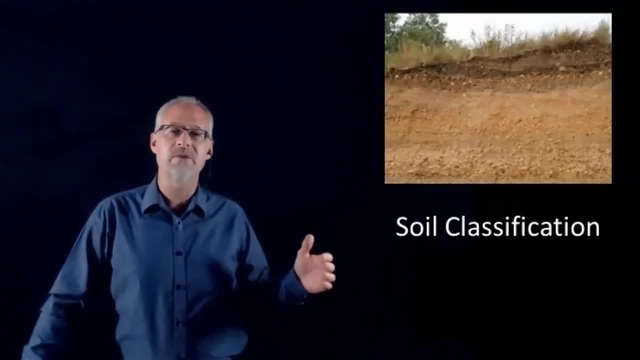 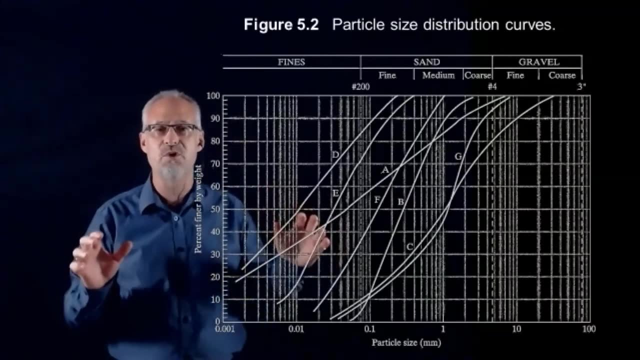 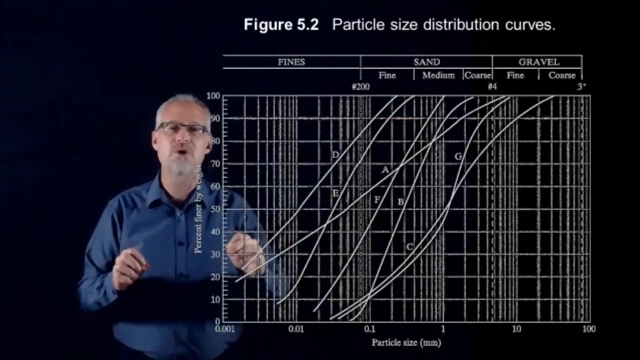 Tonight I want to talk about soil classification. A couple of things I want to point out just as a quick refresher. This is what we call a particle size distribution graph or a particle size distribution curve. These lines that go up and down, these lines each represent a soil sample. So I might say: have a look at soil F, And what I would mean is: look at this line. Okay, right, So this is line F. 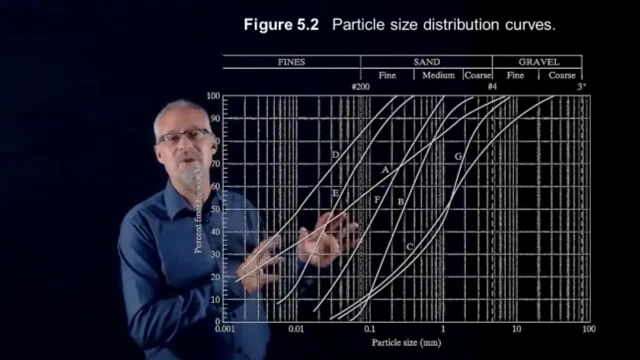 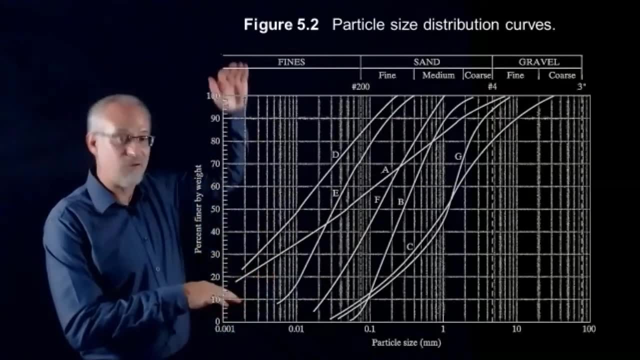 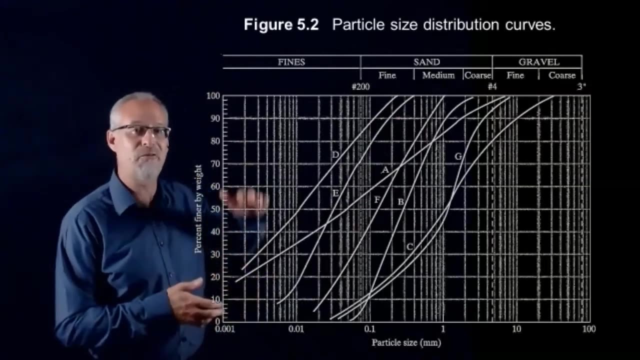 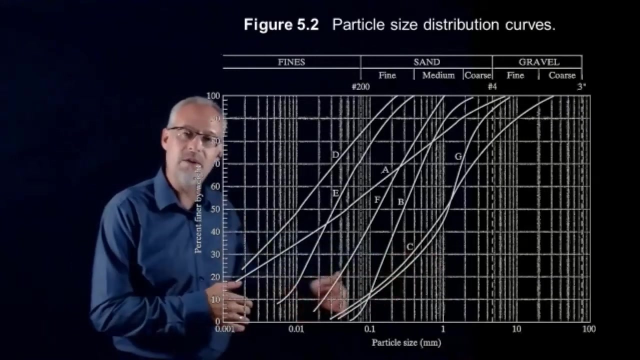 Okay, so that's what those lines mean. The other thing to point out is that this is what's called a semi log plot, where the vertical axis here is a linear scale. That just means a normal scale, And this is percent finer by weight. That's what we do in these distribution curves. But the horizontal axis, that is a log scale. That's why we call this a semi log plot, And you know things to notice. 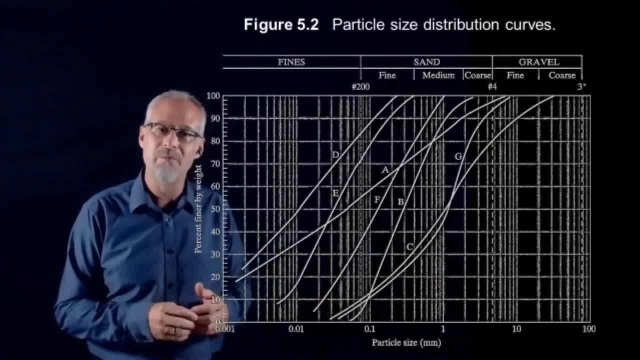 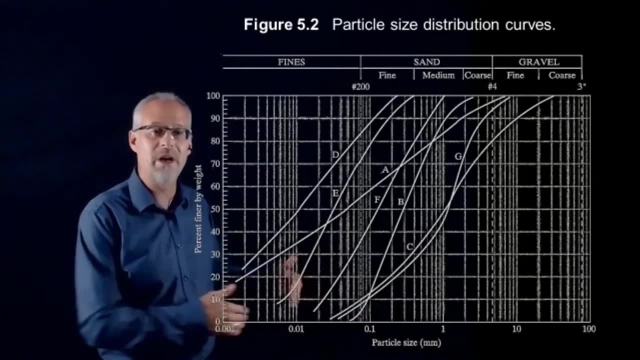 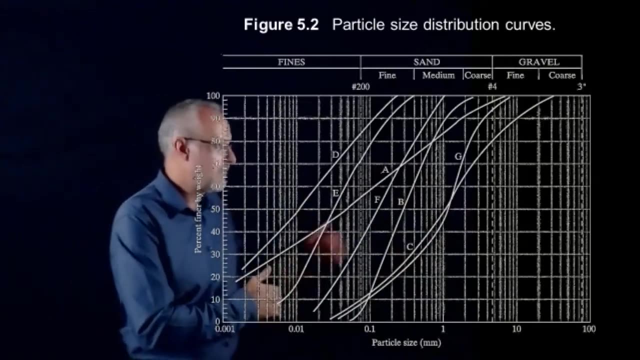 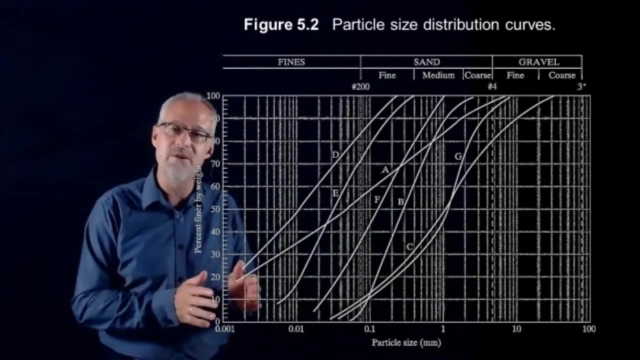 about a semi log scale is that there is no zero. things just get smaller and smaller and smaller. And this is a log base- 10 scale. So every unit is 10 times larger than the next. And because of that sort of scaling of 10 times larger, 10 times larger, 10 times larger, it also means that the intermediate values on that curve are not evenly spaced Right. So for instance, if we go from here: 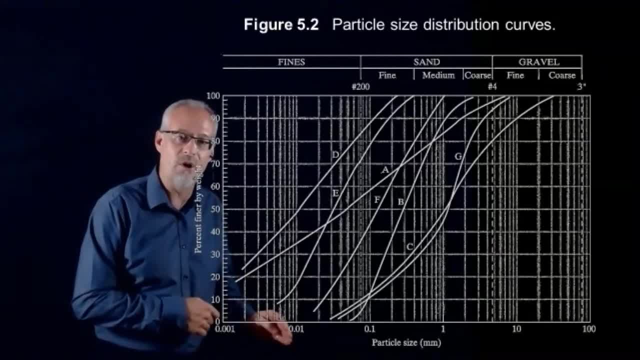 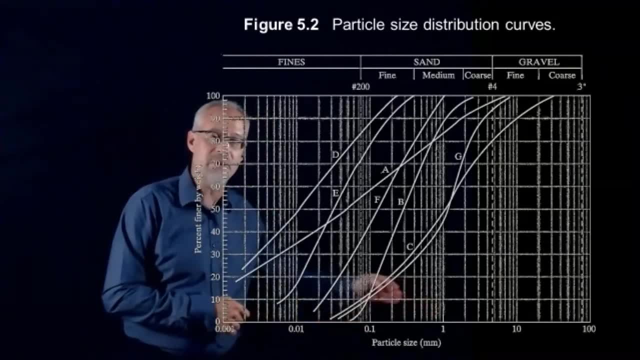 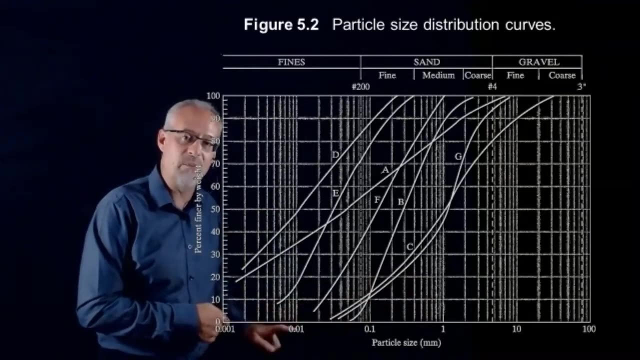 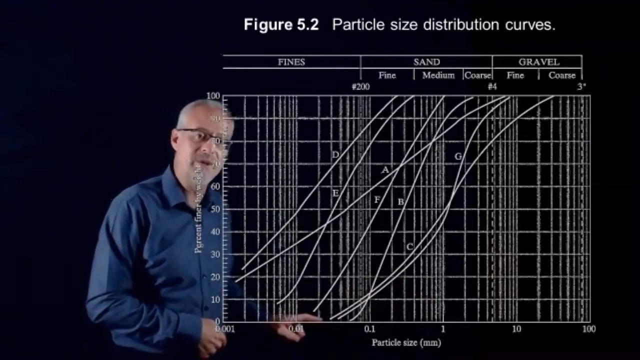 it's point zero one, and then I go to point one, then I go to one. well, well, the size of this division is actually 10 times more than the size of this division, You know. so if this, this point that I'm pointing to right here, is point zero one, then point zero two would be this first line, quite a ways along. point zero three is sort of approaching halfway, And then point zero four is just beyond halfway. So 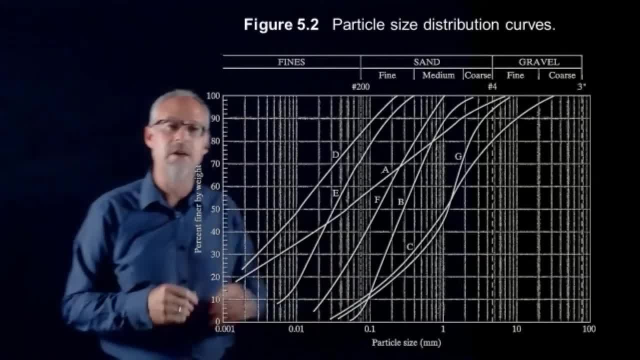 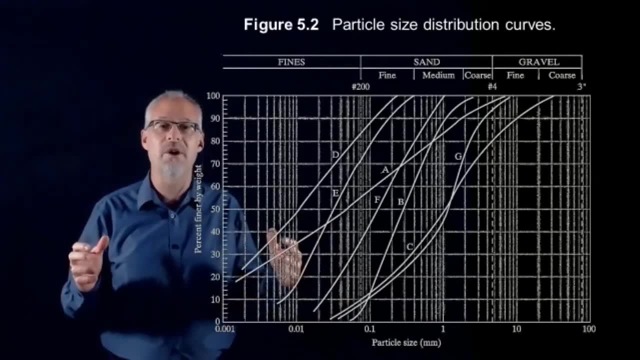 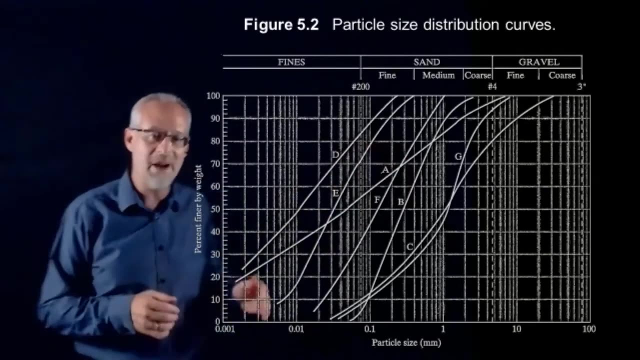 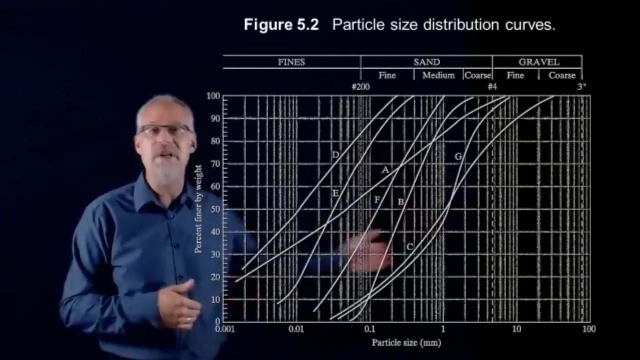 and then the other divisions get tighter and tighter and tighter. that's a. that's a log scale, and the cool thing about a log scale is it allows us to put on huge, huge size differences, right, so we can. we can talk about microscopic particles down here and we can talk about boulders at the other end, but they all fit on one. 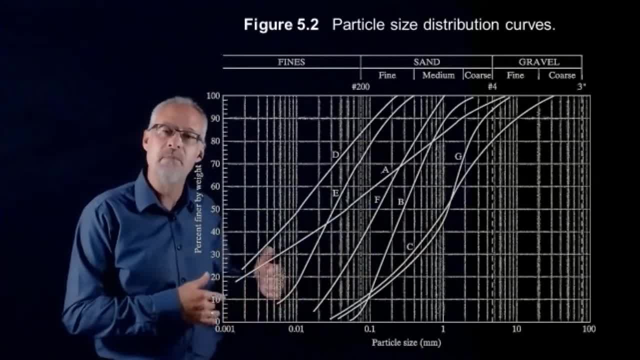 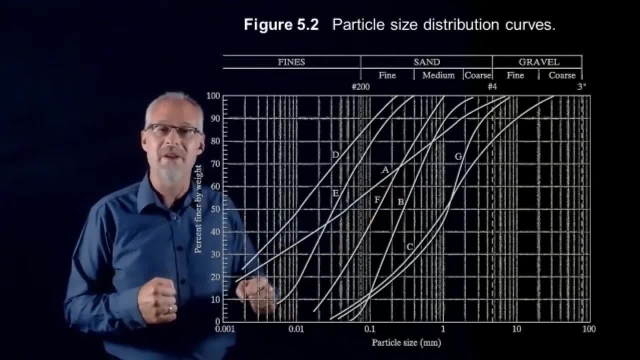 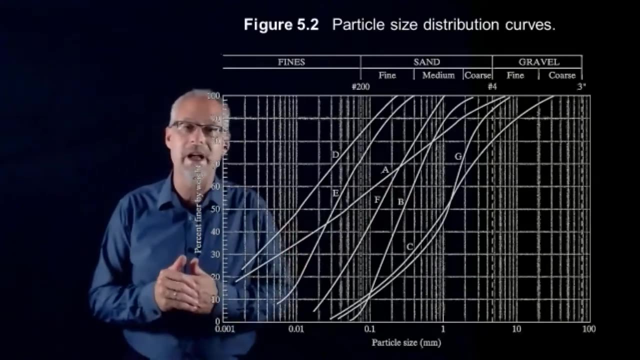 scale and they all have the same amount of, let's say, resolution, even though the scale is gigantic. okay, so it so that the log scale kind of zooms in on the little stuff and zooms out on the big stuff, so that we can see everything, and that's. 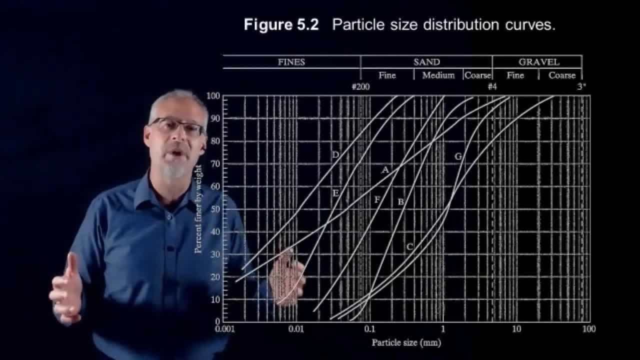 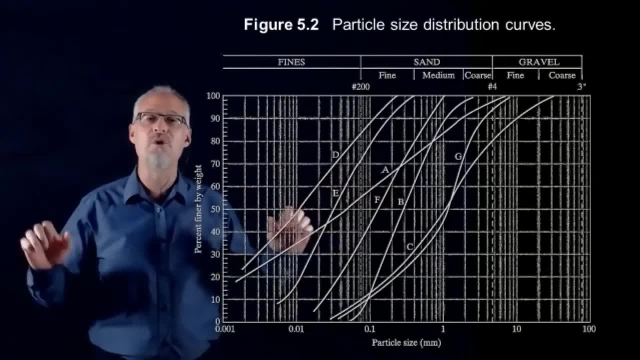 that's very common in all soil mechanics and geotechnical engineering. because so many properties of soils span huge, we call it orders of magnitude. that just means that we have a lot of soil and we have a lot of water and we have a lot of things like ten, a hundred, a thousand, ten thousand. those are orders of magnitude. 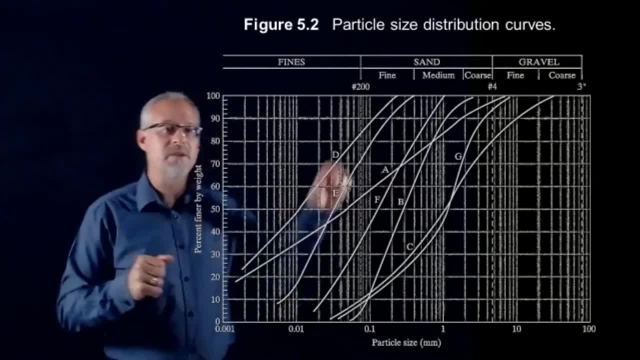 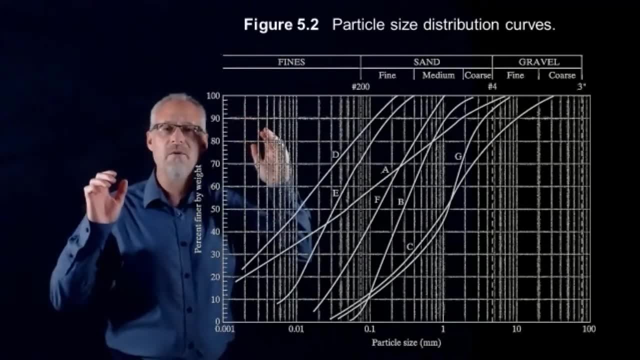 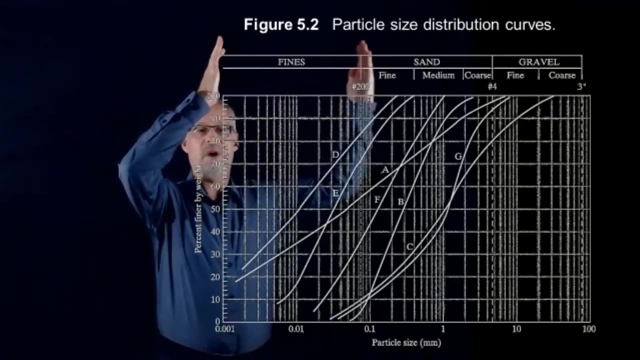 fancy word. the other thing I want to point out is on the top we superimpose this scale that tells you where, where things start. okay, the small stuff is that down at this end. so here we call this the, the fine grain soil. remember, soil is either fine grain or coarse grain. fine grain stuff is here and the 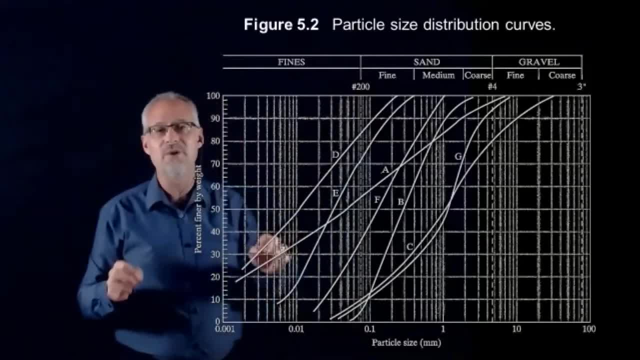 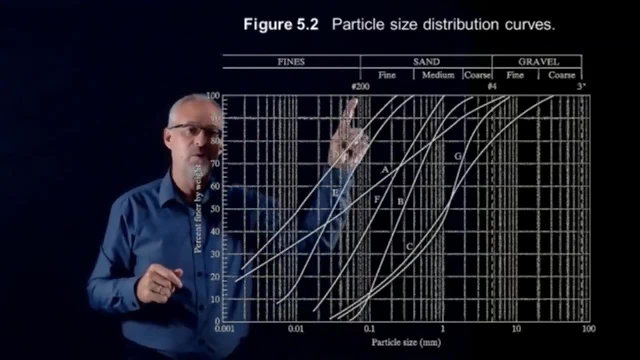 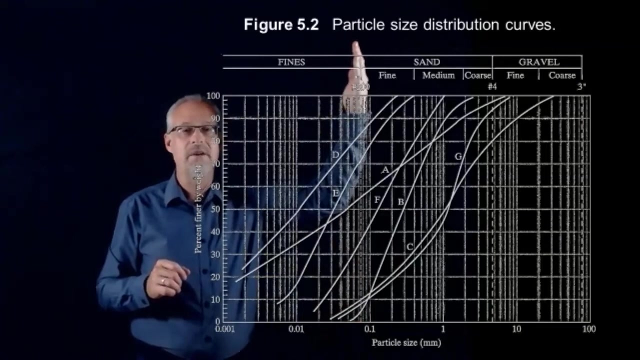 division line is the number 200 sieve, which corresponds to point zero seven five millimeters particle size. so if you, actually if you, followed this line all the way down, you'd find that it goes, it's, it crosses somewhere in here, which is point zero seven five millimeters and that's, and this is where we define silt. 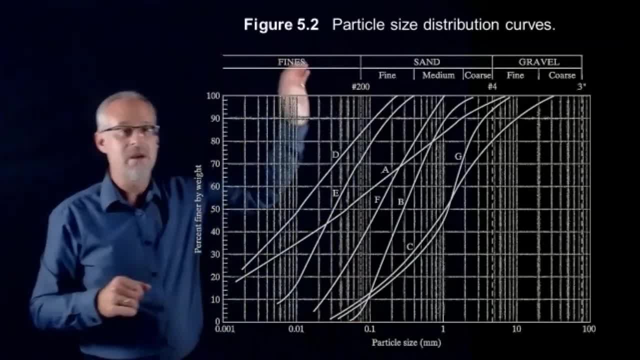 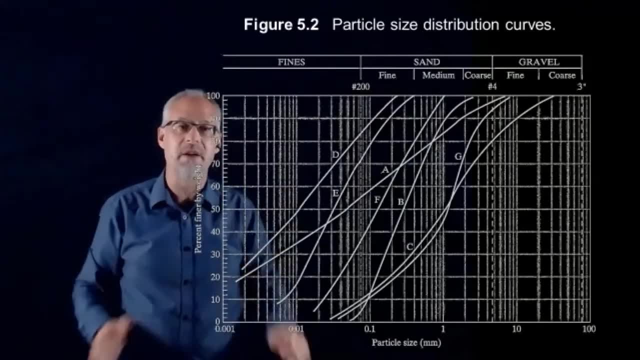 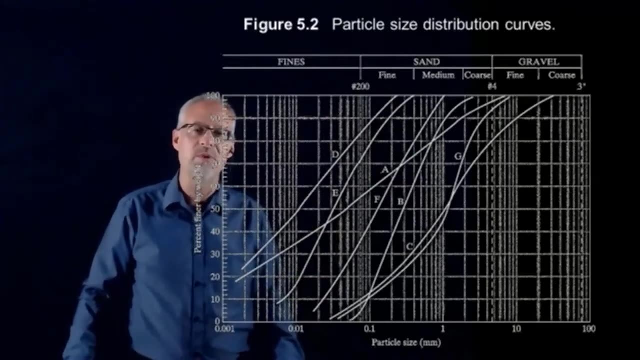 and clay are on these sides, and then you can see sand and gravel and the number four, sieve, is the division sand and gravel. that should be just a nice quick refresher. someone says: why do some of them not start from zero percent? good question. so you'll see these lines like: 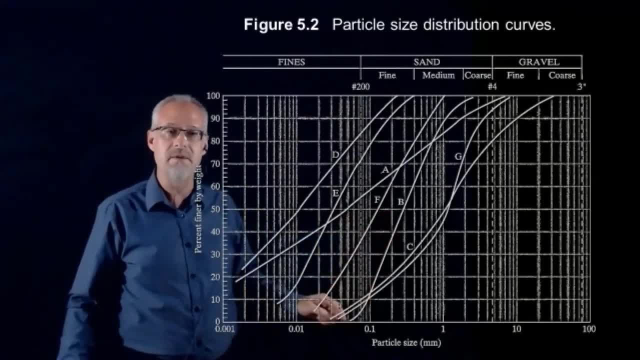 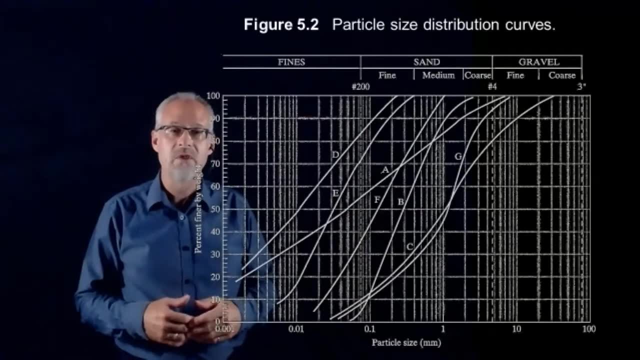 some of these lines go all the way down to nothing, and what that means is that if there was a sieve test done on soil sample B, it means there was hardly any dust left passing the the number 200 sieve. it was just a tiny amount and they were able to just give one point and say wow. 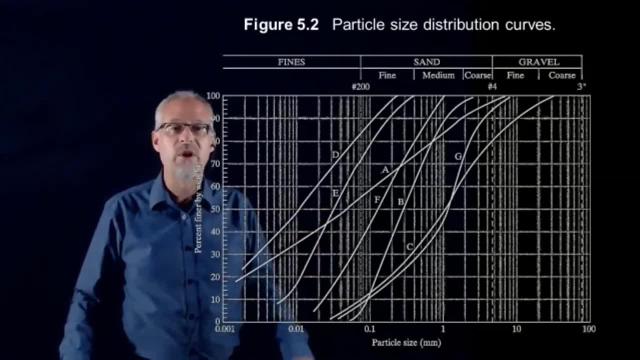 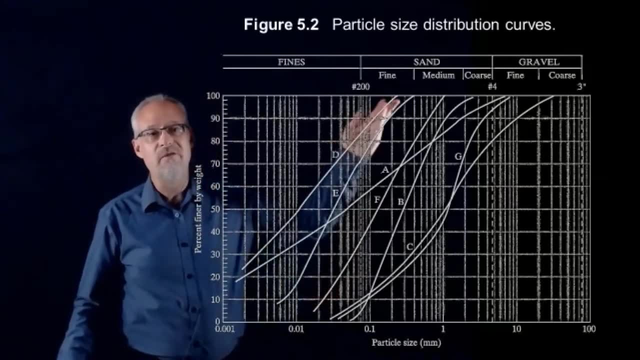 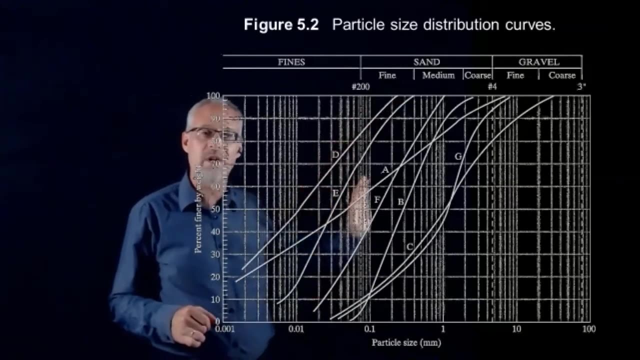 we've accounted for the entire sample. we'd look at something like soil b and we would say it's very clean, something like soil d. we've done a, we've we've done a test and we did a. you have to do a hydrometer, right? so remember, the sieve is what is what we use for the coarse grain soil. 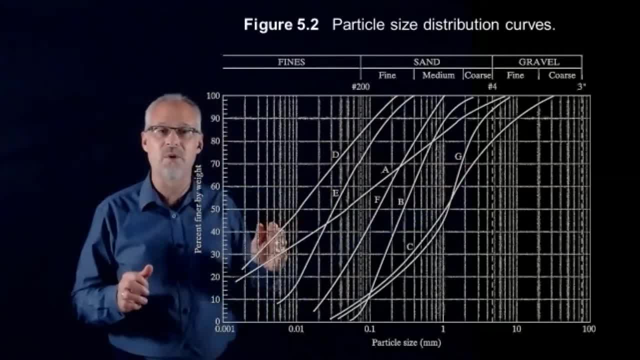 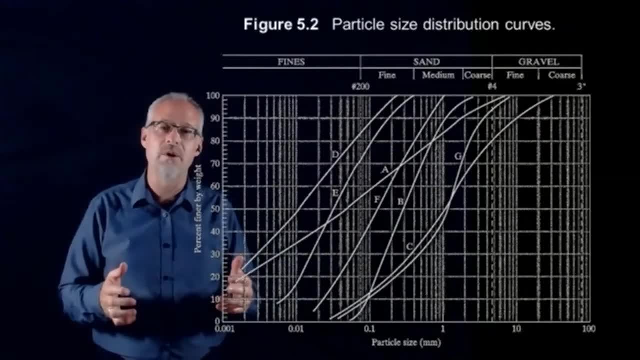 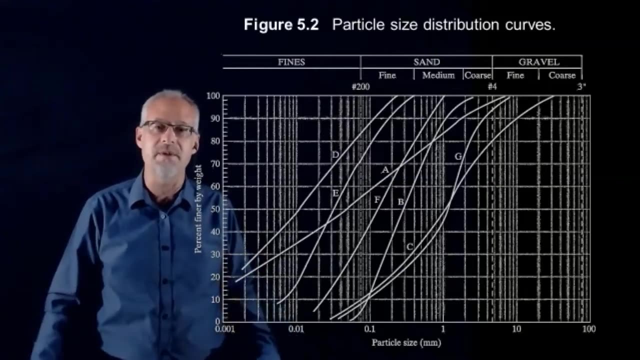 distribution data and then the hydrometer is what we use for the fine grain soil. that's where we let the soil settle out of suspension. i'll tell you what. there's some soils that would take. that takes so long for the particles to settle out of suspension that people just stop the test and 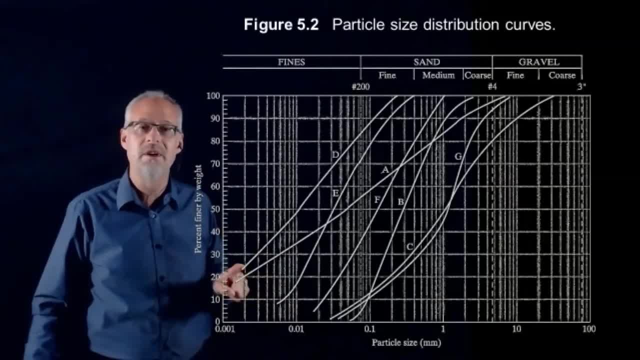 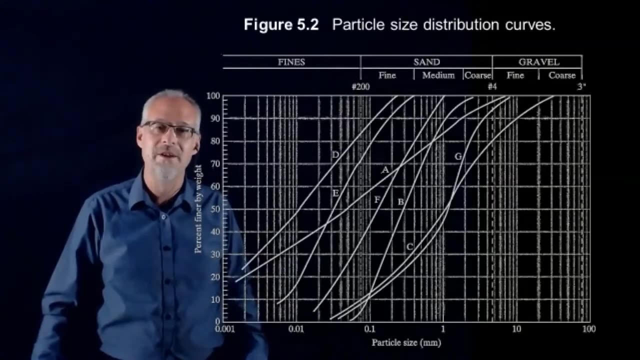 they say, well, okay, this. this is our last data point and all we can tell you is that there's a whole, there's 20 percent, 22 percent more of that soil. that was still in that that solution, that we just kind of didn't have time or patience to figure out what was in it. so 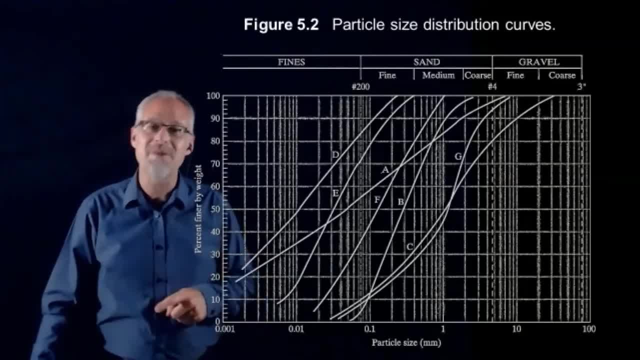 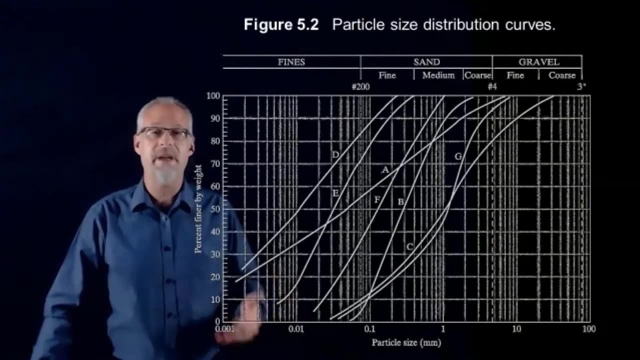 so there's, there's, there's more mass, but it was still left in the soil suspension and maybe they left it for a few days and it still hadn't settled out. it just means that there's tiny, tiny fine particles floating around in there. so where these lines stop is kind of where the test stops it. 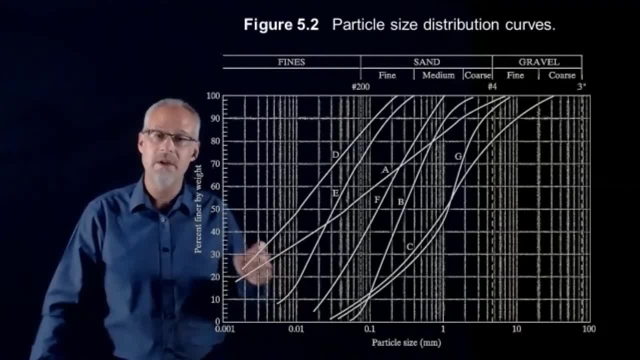 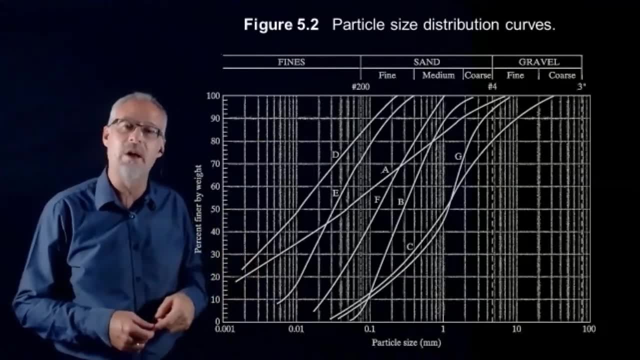 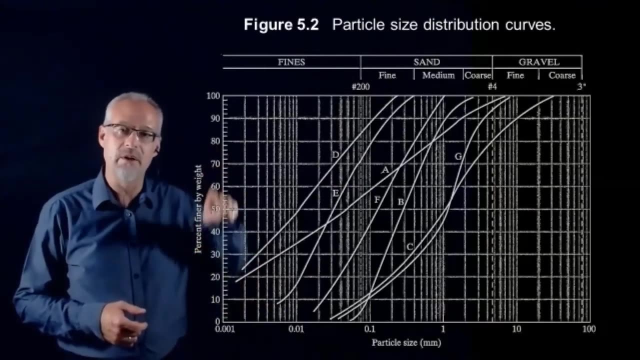 doesn't mean that the sample doesn't exist. it does. it actually has to right. so these lines. it's quite reasonable to be able to extrapolate these lines and say: well, we know, we know that that 22 percent is definitely finer, because this, this, this, uh axis says percent. 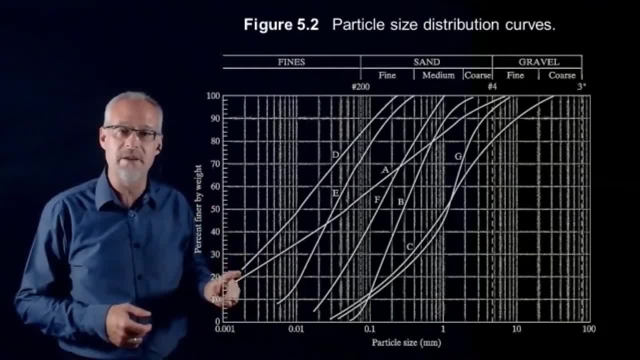 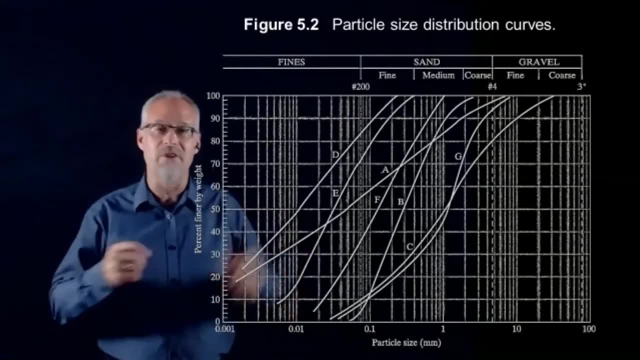 finer by weight. so there, what you can say is that 22 percent of of soil d was finer than 0.007, or something like that, and and so that it's just where the test ended. that's, that's the answer to your to your question, but it's a good question. 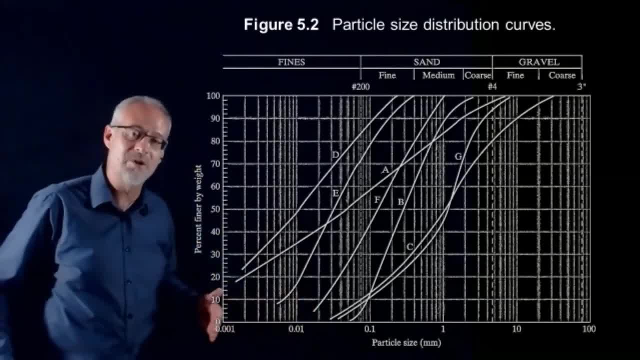 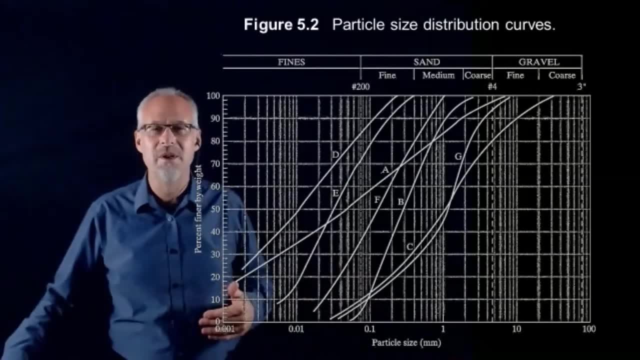 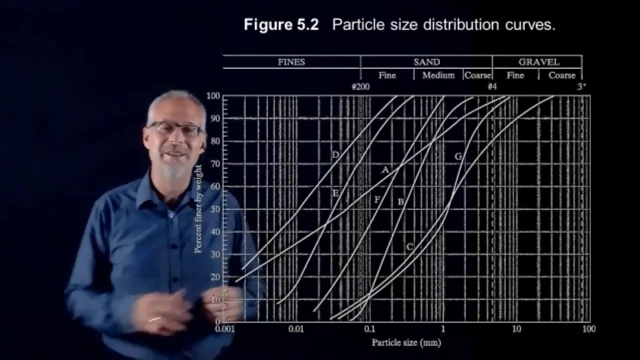 also note that, remember, this log scale doesn't doesn't ever go to zero in terms of size. and you think about it. that makes sense, because what is a zero size particle? I don't know? is that like a black hole? I don't know? so it's a singularity. I guess that's what it is. so for particle size, it 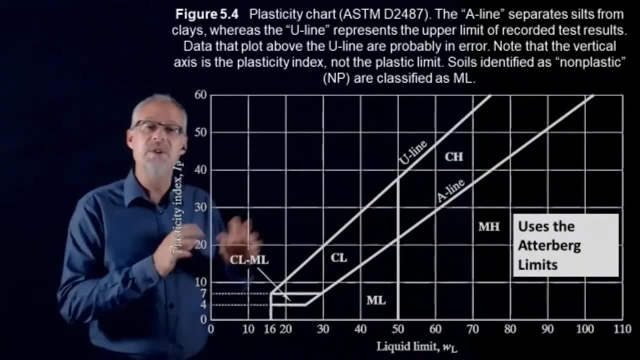 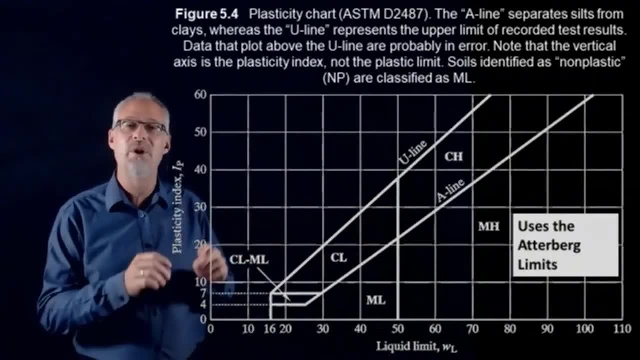 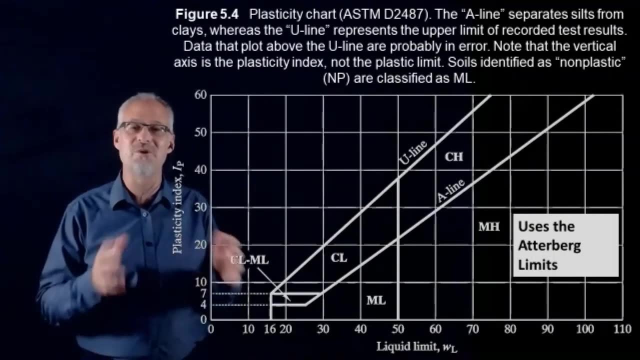 kind of makes sense for us to use a log scale. this is the plasticity chart and we this actually shows up in your Atterberg limit lab write up for how you classify the type of fine grain soil that you're testing, and it's what. it's the plot of your plasticity index. right, so your plasticity index. 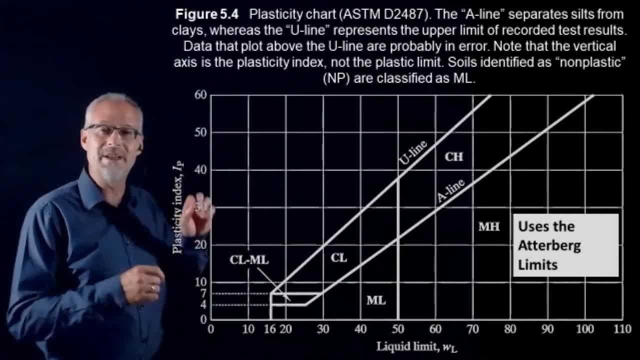 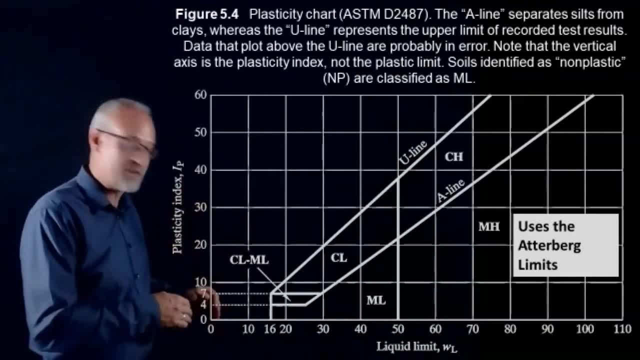 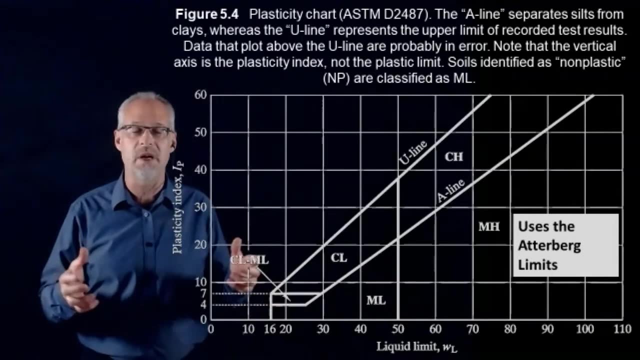 is on the vertical scale. the plasticity index is the liquid limit minus the plastic limit is the plasticity index okay versus the liquid limit. and what you do is when you, when you finish your Atterberg limits testing on a soil sample, you plot a point and the point will fall somewhere. 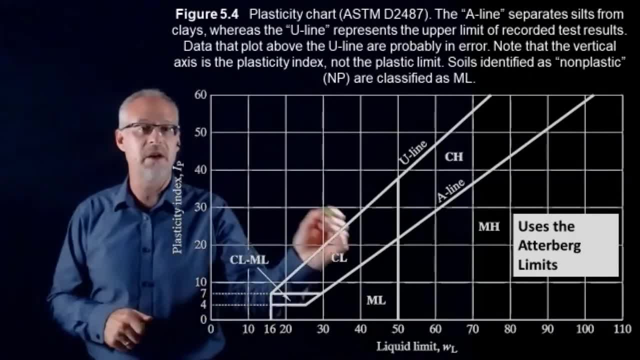 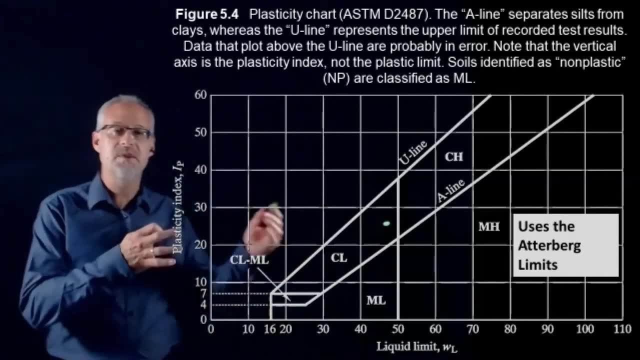 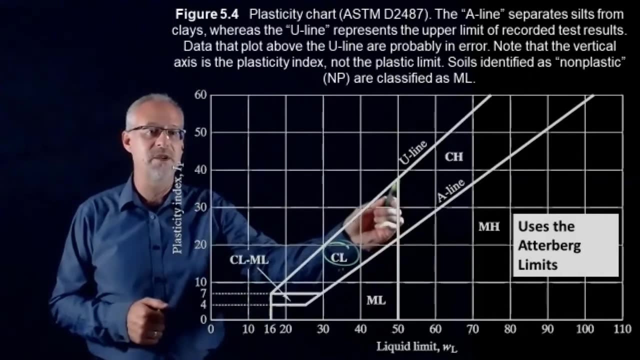 maybe the point you know, I'll draw it so. so let's say, let's say the point falls, falls here from your lab data. what that means is this soil is a CL. okay. so if the because it falls inside, you see where the thick lines are. there's kind of a funny trapezoidal shape. 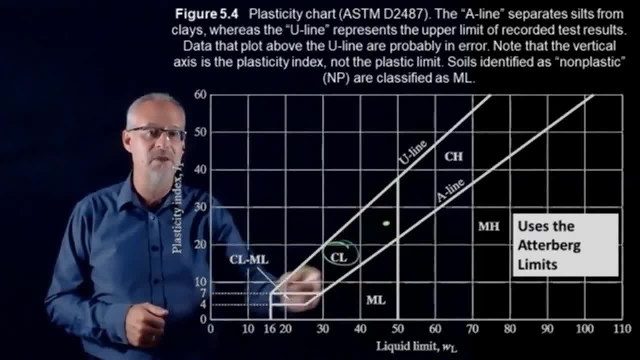 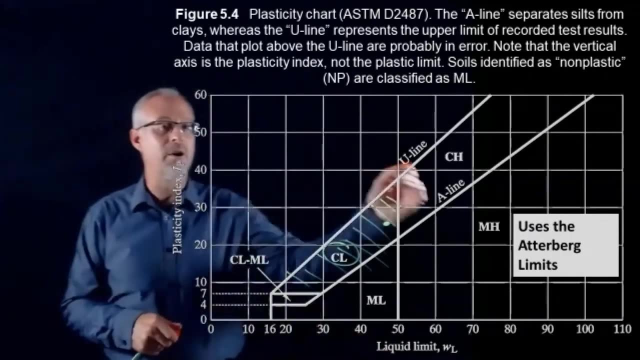 and if, if your dot falls anywhere kind of in this region, that's going to be a CL. I mean, if I was really good I could, that's not bad, okay, so that region, that's all CL. similarly, you know, if you're, if you plot up here somewhere, that's going to be a CH. plot down here it's an ML, over here it's an MH. 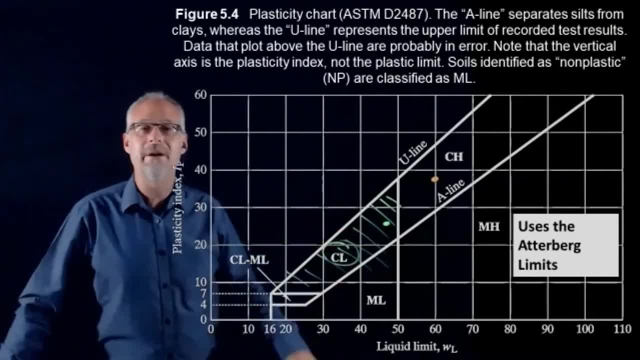 um, yeah, someone said: well, what if it's, what if something's on the border? ah, that's always always a problem. um, you know, it's, it's unusual. you'll get something right on the border. and if you do find something on the border, you could always go back to this, the hydrometer- and say: 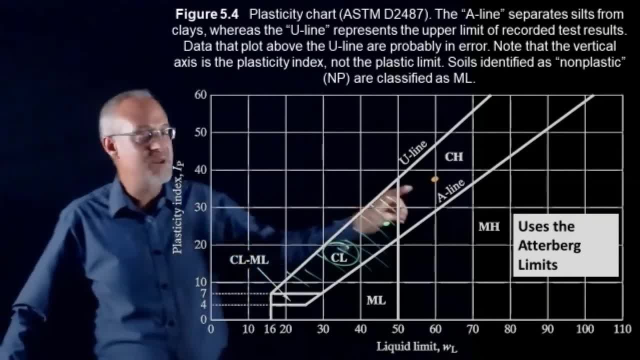 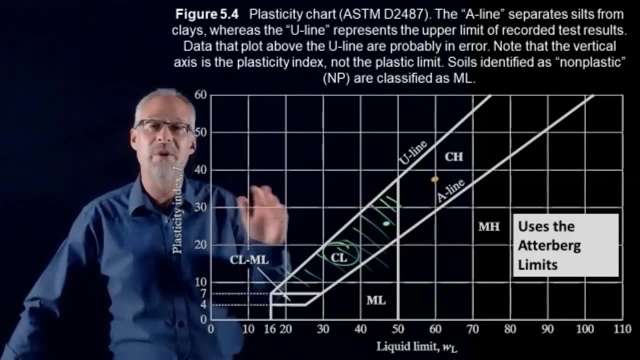 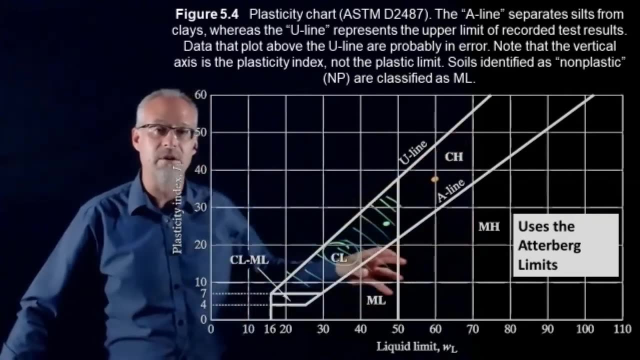 what the percentage is. because I'll tell you what this, this a line. the a line is the theoretical, or actually it's not really theoretical. it's sort of experimentally derived division between clay right here and silts. the silts are down here, okay, so so there's, there's a, there's also funny spots, so 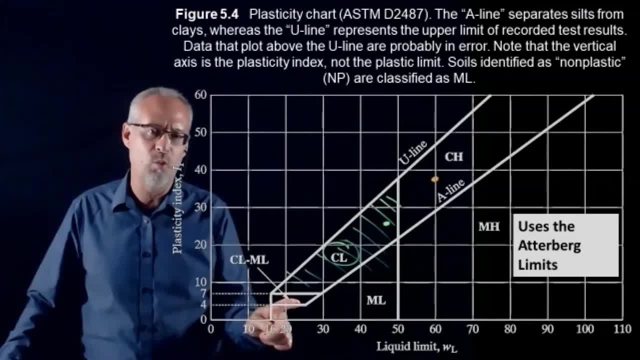 it's a good thing to point out if you happen to have a soil that's down here. this is a funny little tiny region and it is possible to get soils in this region where you would give them a different two-letter code. and let me just define what these letter codes mean and this: 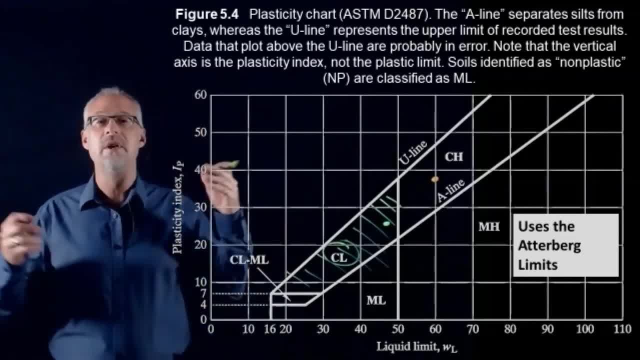 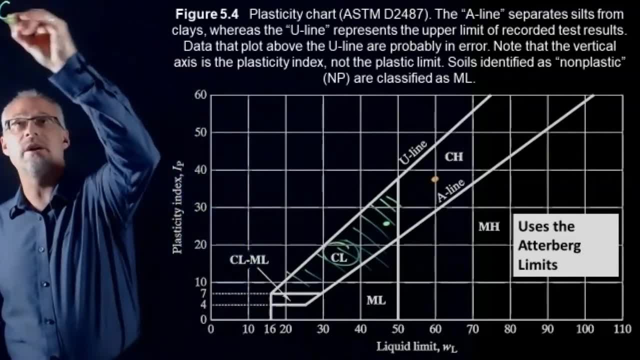 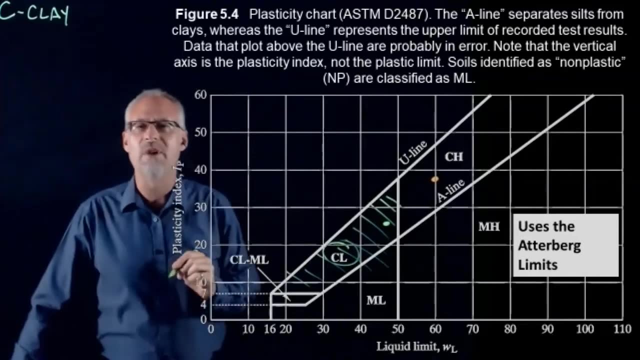 is kind of the beginning of what we're doing tonight, uh, surrounding the the unified soil and two-letter code system. so in the two-letter codes, uh, we're going to use the letter C and we're going to use the letter C to indicate clay. okay, I know I'm right on the border there. I'll. 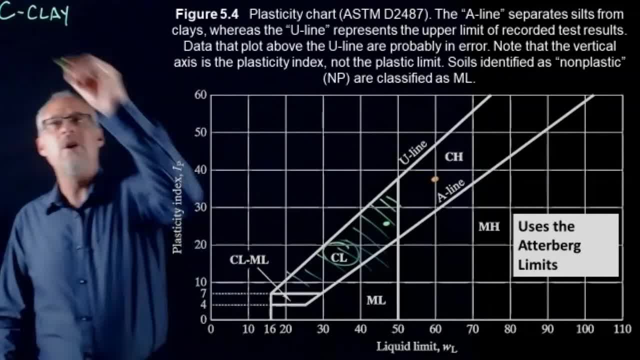 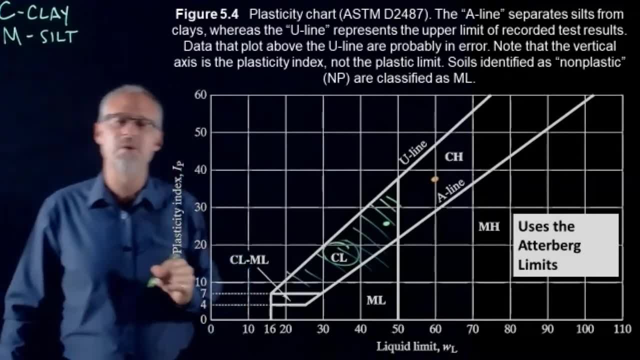 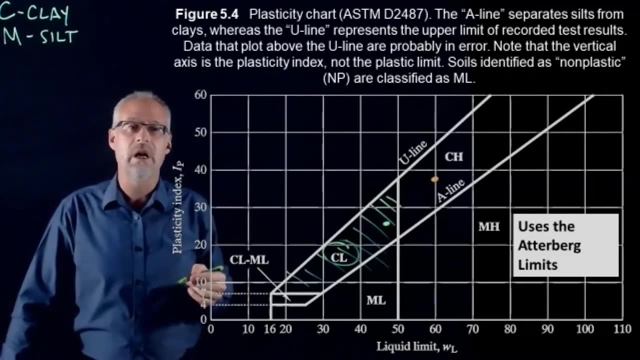 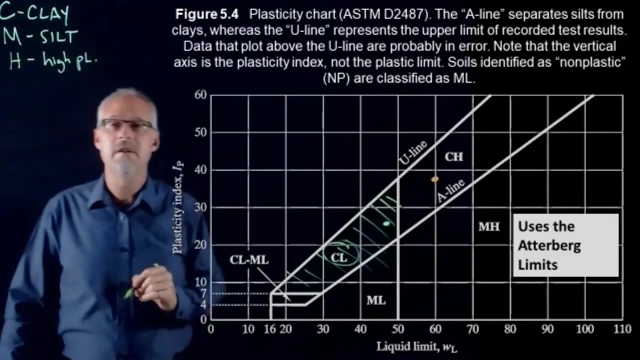 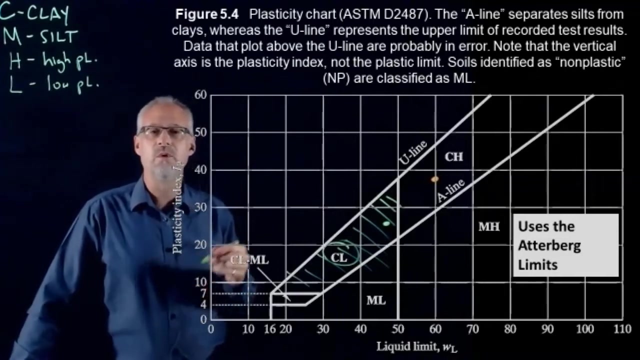 move a little bit. so C means clay, M means silt and I think S doesn't mean silt because S means sand, which we'll get to later. so S was already kind of taken. so we use M for silt um H means high plasticity and L means low plasticity. okay, so so we'll we'll for fine grain. 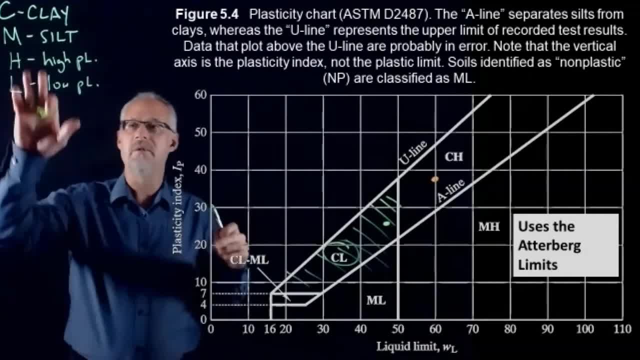 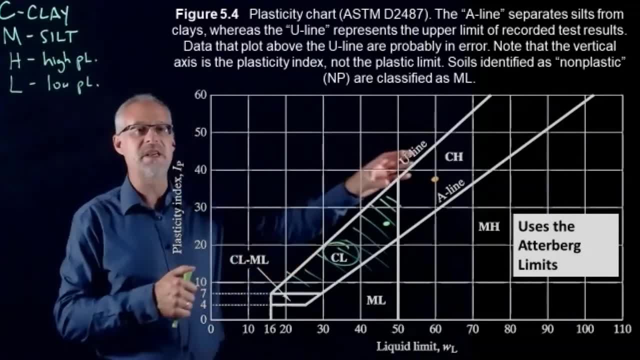 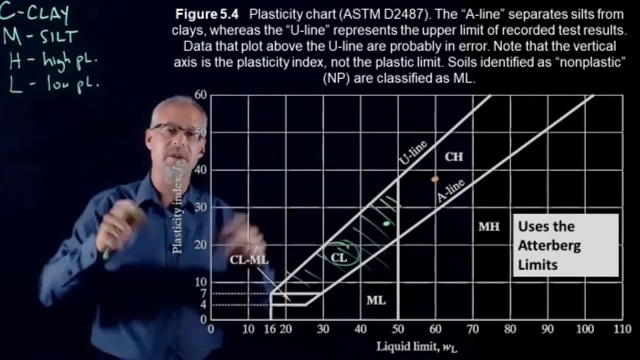 soils, these sort of letter codes, uh, have these these meanings? okay, and we'll so if you, if you look at this and you say, oh, we've got a, we've got a C H, like a C H is a high plasticity clay and M H is a high plasticity silt, Etc. Etc. okay, so that's what those mean. on, 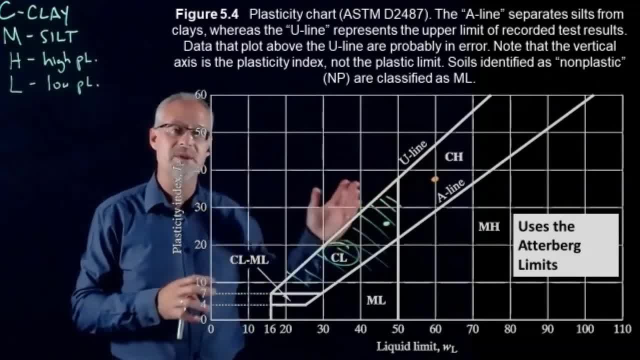 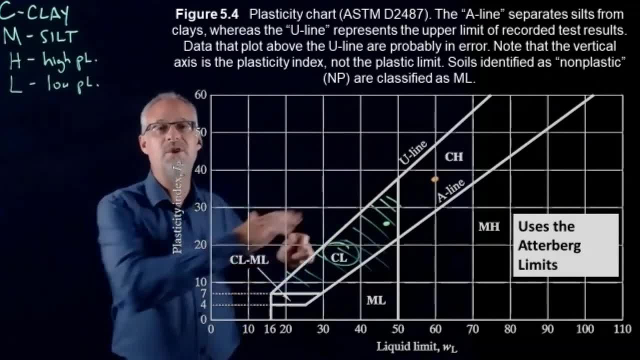 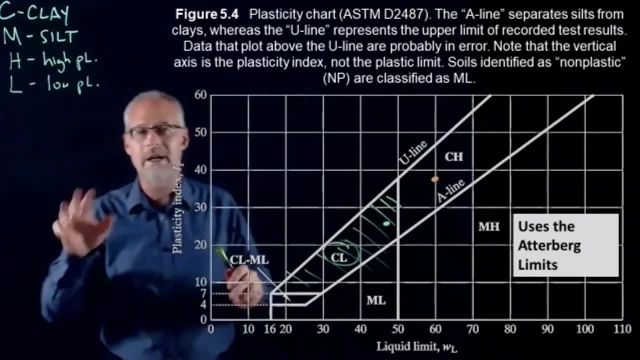 this curve. the A line, like I said, is the division between silt and clay, C's and M's, and the U line is sort of um, we don't observe values above the U line. the U line is kind of like: if you get a number above the U line, uh, maybe you made a mistake doing your lab and you better go back. 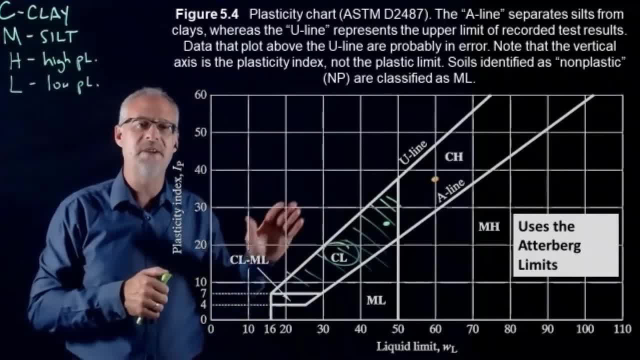 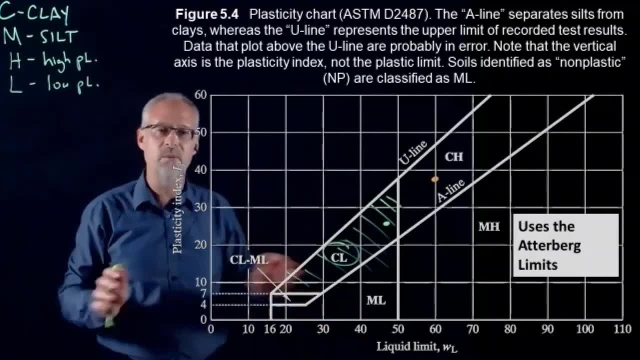 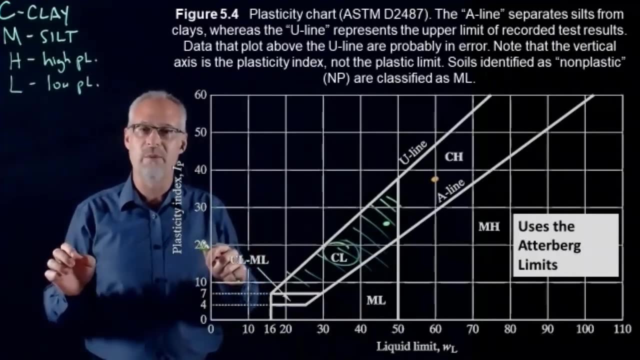 and check it, because you know, properly done tests do not plot above the U line. so that's, that's what that means. and I'll just a quick note too: the liquid limit and plastic limit, those are a number, but the number is actually the water content, and I hope everyone remembers the formula for water content, right? so 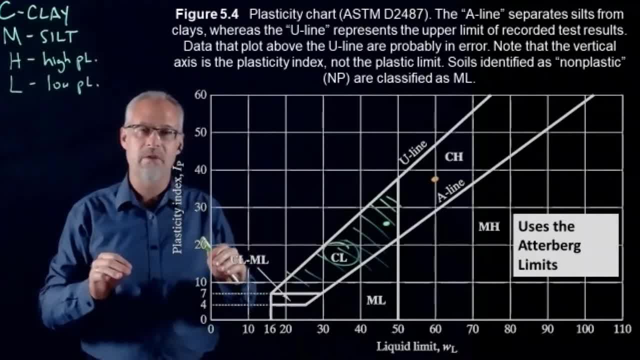 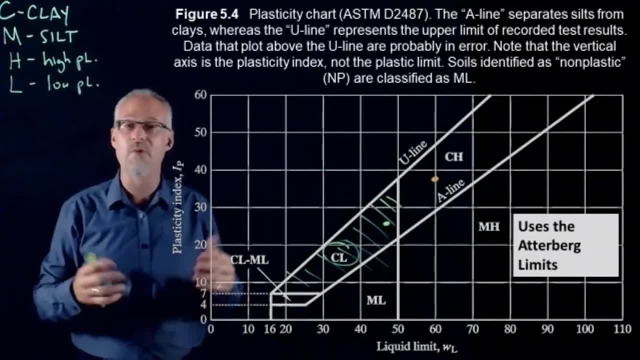 mass of water divided by mass of solids. right, so. so even though we express it as a kind of percentage- I said last class- it's really better thought of as a ratio. it's a ratio of the mass of water to the mass of solid, or the weight of water to the weight of solid. same same. 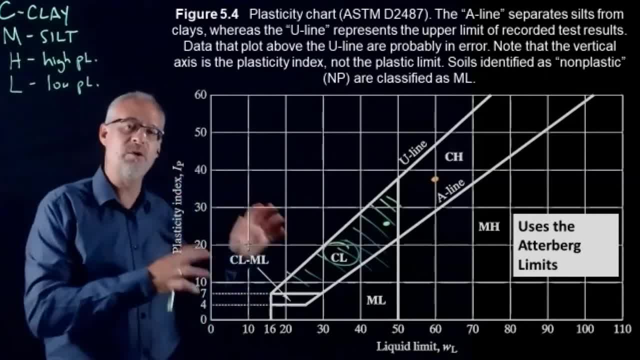 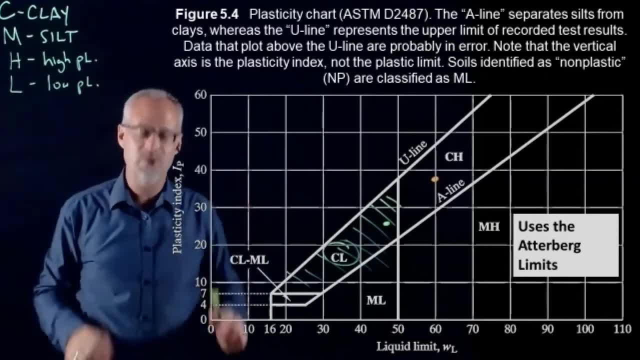 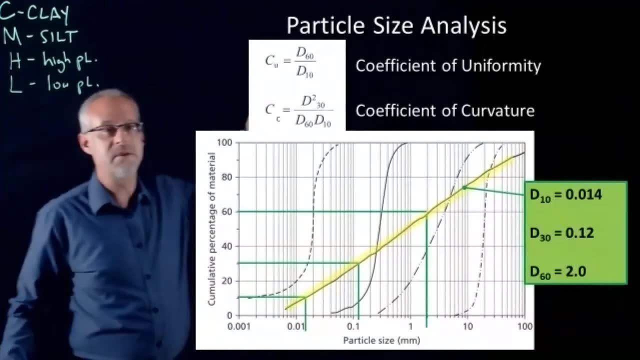 thing. okay, so that's that's, uh, that's how we use the Atterberg limits to determine, uh, these two letter codes that we're going to get into a little bit more more tonight. okay, the other thing I wanted to sort of refresh your memory on was these two uh, C, C, U and CC. that's the coefficient of uniformity. 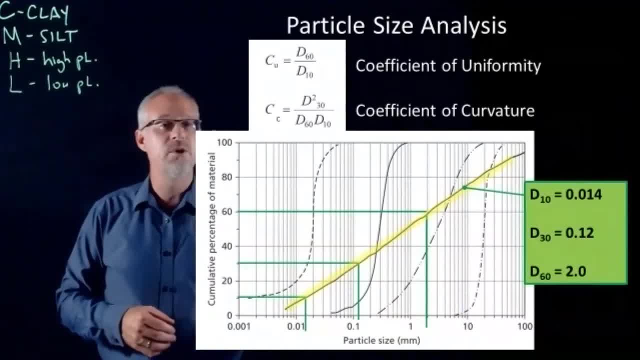 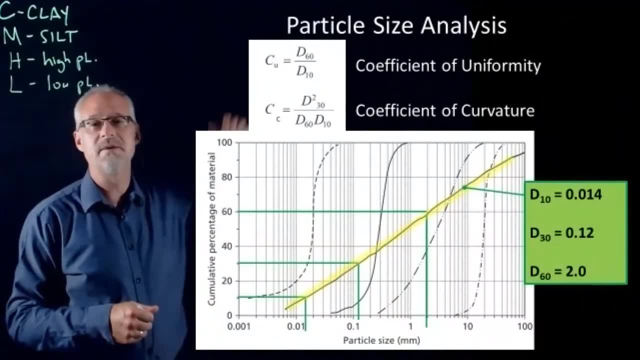 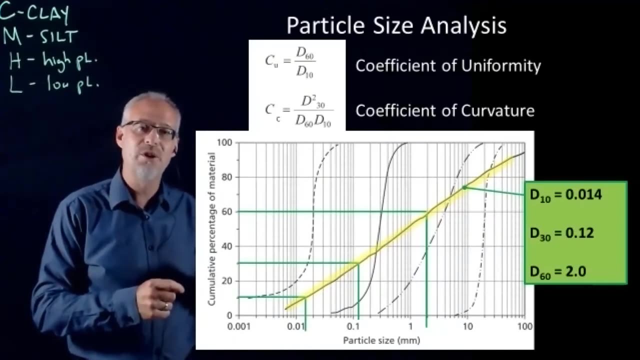 and the coefficient of curvature, and for these two um, for these, these two, I guess, formulas- for lack of a better term. you need to be able to read off the- the diameter at which, um, the curve for the soil crosses either the 10 passing, 30 passing or 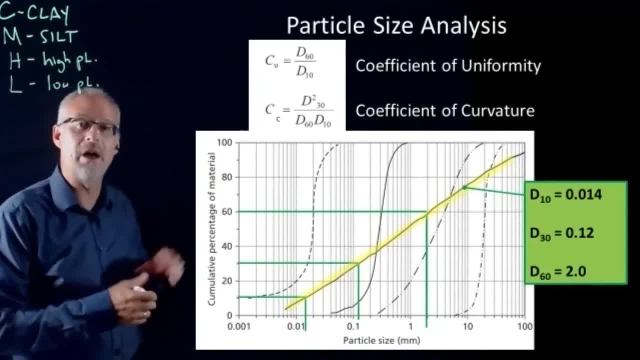 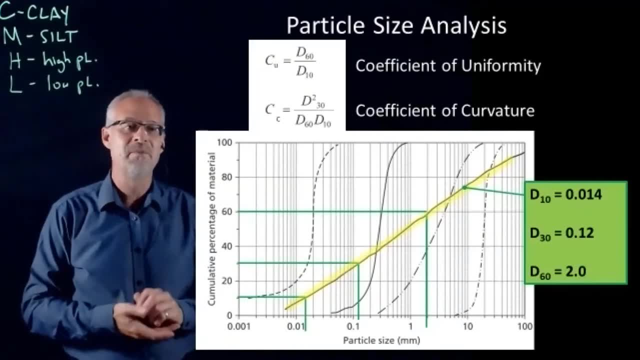 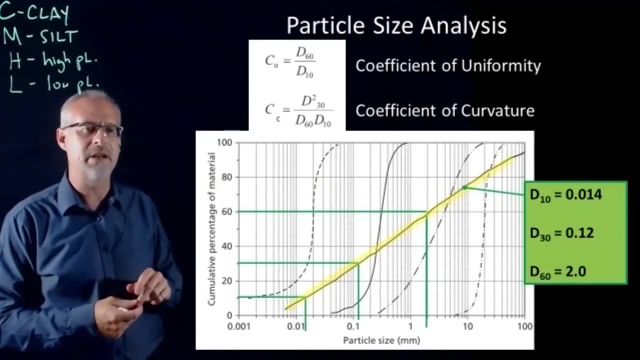 60 passing and that's indicated by these, by the green lines on this curve. you can't see through them because I just copied this from last week's slides. but just as a sort of a sample I put some of the numbers, I think the d10. we kind of debated a bit and maybe the d10 should be 0.013 or 0.012. 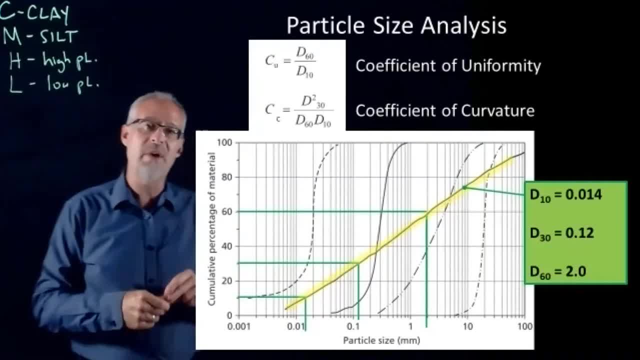 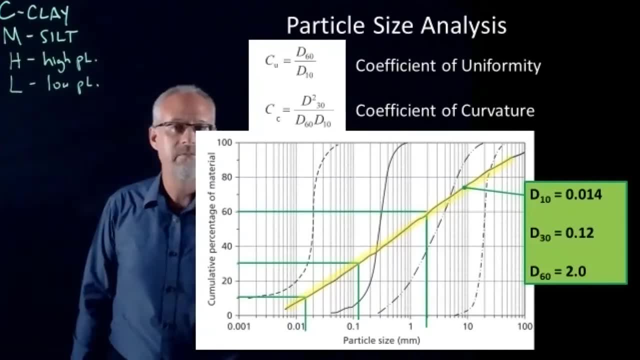 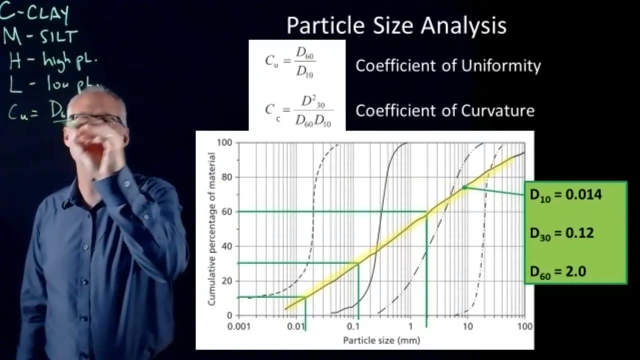 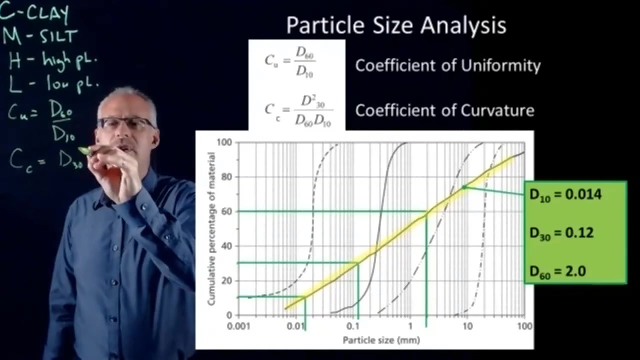 something like that. I can't remember, um, but uh, but basically we're going to need this for what is also what's coming later. I might even just jot them down, you know, put them over here. so just remember that C? U coefficient of uniformity is d60 over d10 and uh, coefficient of curvature is d30 squared over d60. 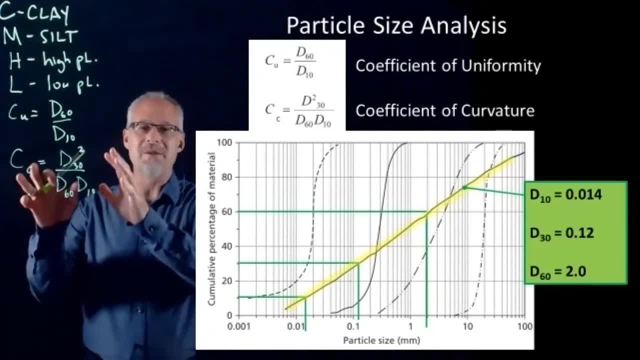 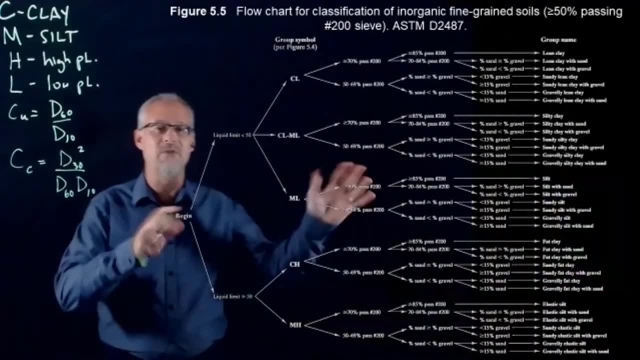 times d10. okay, so this is. I'm just collecting the things that we're going to need. um, so, the first thing now: now I, I, you can't read this. I, I can't read it, but I'm just. I zoomed back out on this, uh. 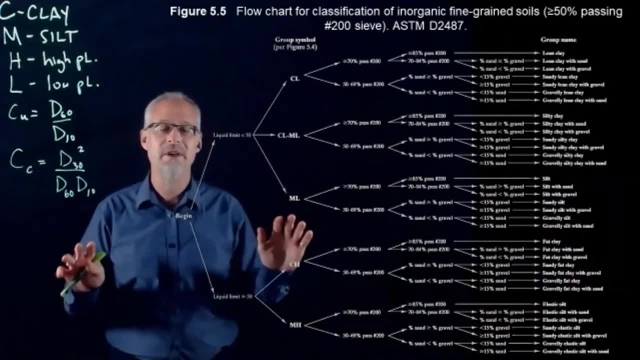 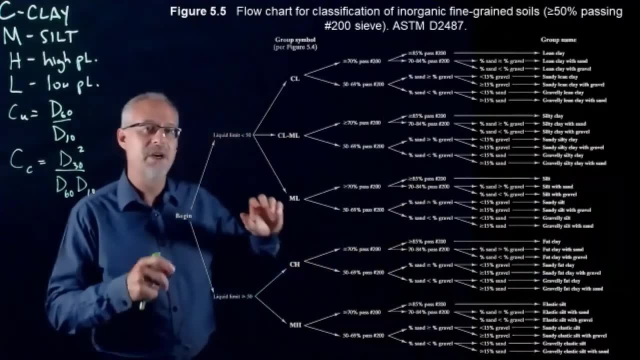 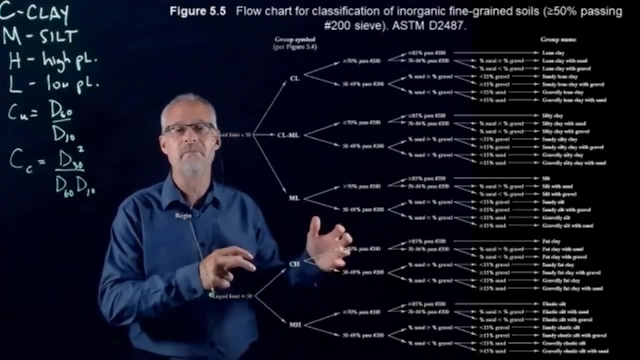 this flow chart because this is what I want to actually work on tonight. one of the things I want to do tonight. this kind of complicated Chart is the chart for classifying and giving a what we call a group name to a soil sample, and this particular chart is for: 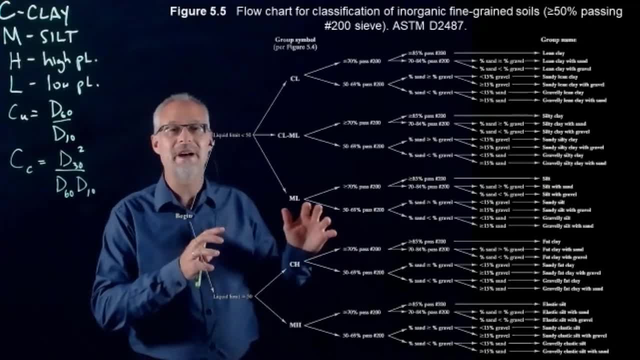 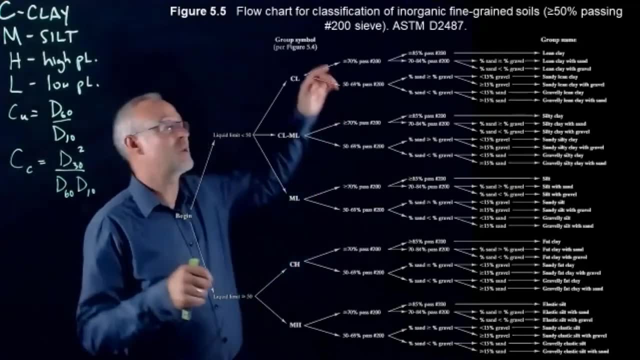 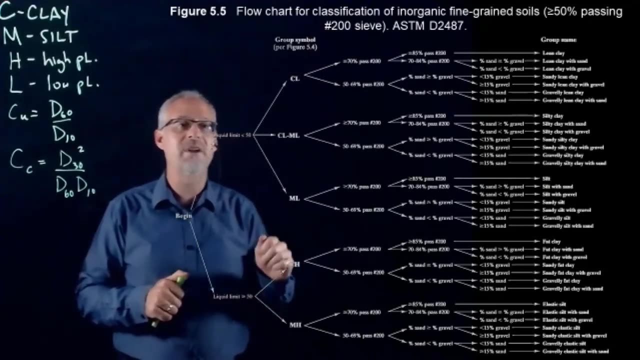 fine-grained soils. okay, and how do we determine if something is a fine-grained soil? and the definition is actually it right up here in the name of the chart. so it says flow chart for classification of inorganic fine grain soil and in brackets it says greater than 50, passing the number 200 sieve. 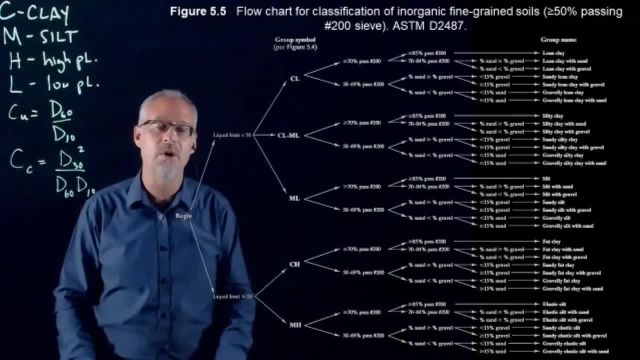 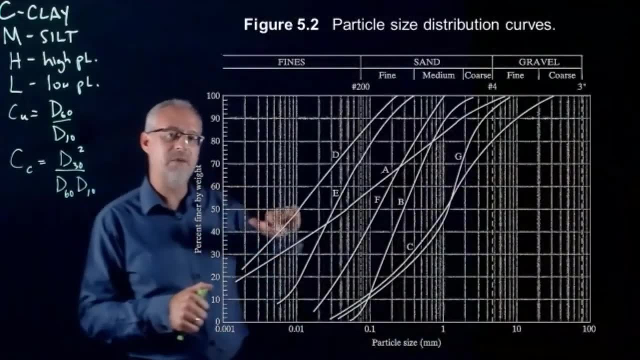 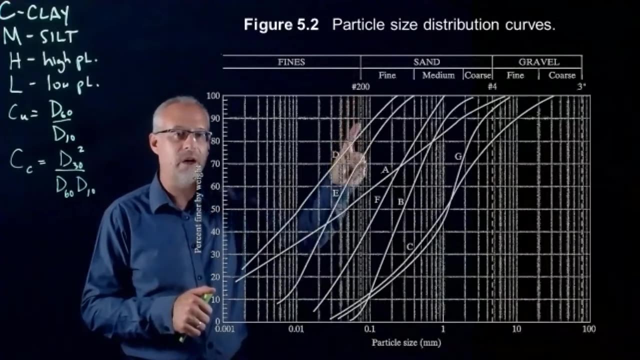 so in essence, the definition of a fine grain soil is something that, if i look at the at the the curve for that particular soil sample, and i look to the number 200 sieve cut off and i come down here to 50 percent, it looks like i have three soil samples. 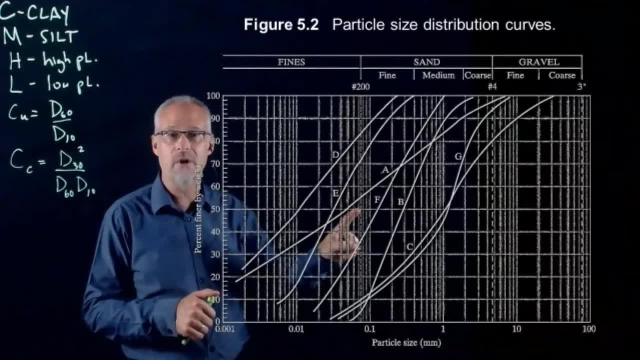 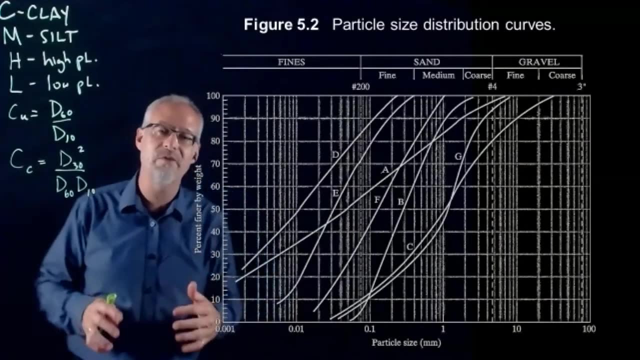 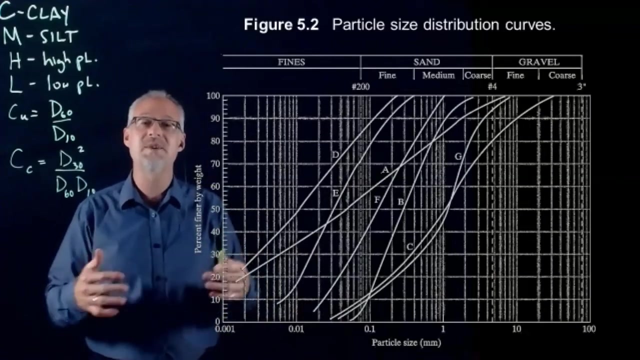 that are that have a line above 50 percent at the number 200 crossing line. so soil a, soil e and soil d appear to be all fine. what we would classify as a fine grain soil- and that's the first lesson in tonight's classification- is to how do we decide if it's a coarse-grained or a fine? 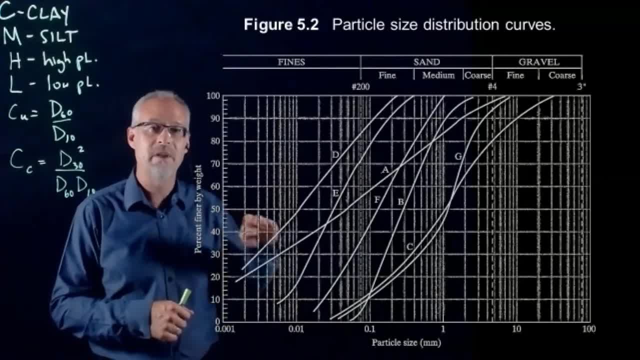 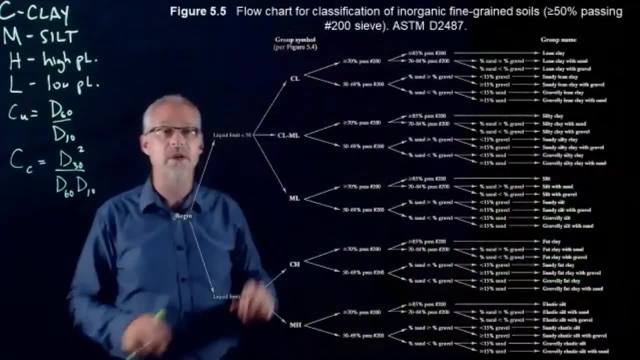 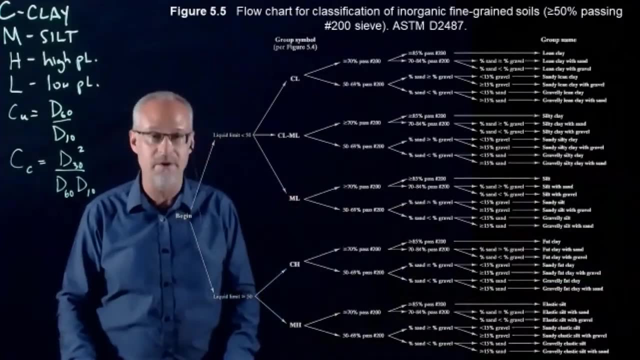 grain soil and it's really that 50 percent line combined with the number 200. okay so, and we would classify them using this particular flow chart. okay, and we'll go into. there's some nuances to this flow chart that we'll actually get into. so first, well, so first assume that we're going to 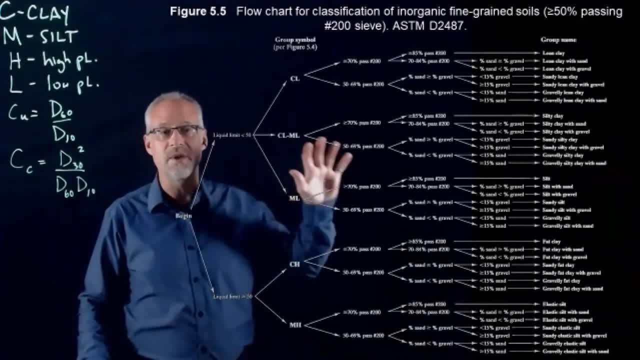 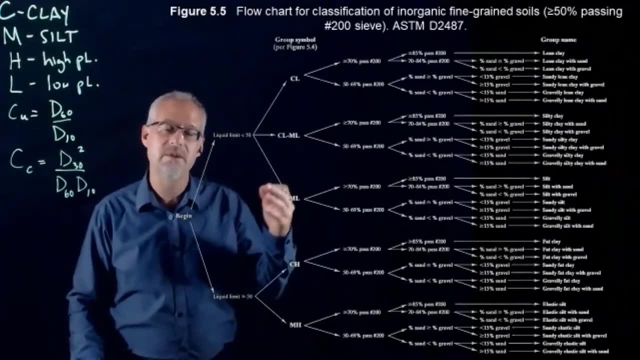 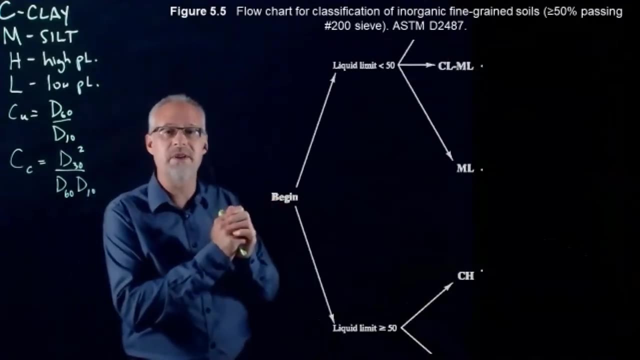 look at the classifications of the soils, because they're the only ones that would apply to this: the classification of so-called inorganic fine grain soil, basically silt and clay. so the first choice that we have- and i think you can read this- the first choice once you've identified the soil. 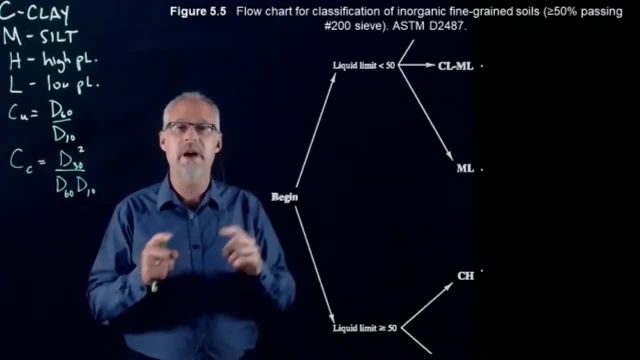 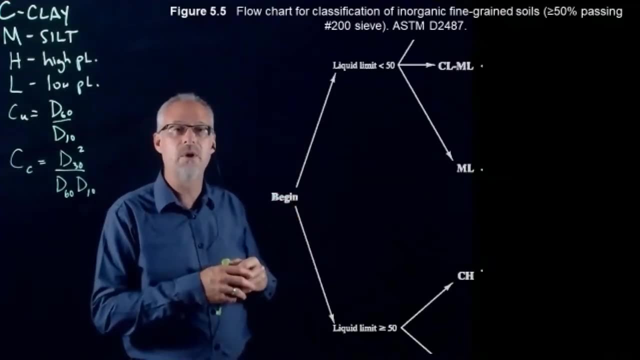 as fine grain is. we use the liquid limit. we use the liquid limit as the deciding factor for the first decision in this classification soil. so you can see there's a lot of different choices here, so we'll start with this one. the liquid limit is a very significant change in the population. 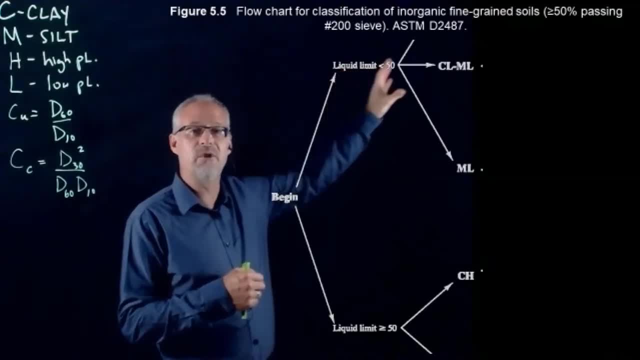 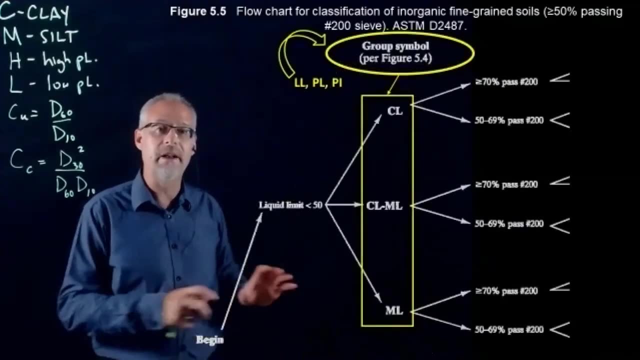 system. so if our liquid limit is- let's just say, hypothetically our liquid limit is- below 50, then we're going to follow the the flow chart in this direction. otherwise, we follow the flow chart in this direction. okay, not too difficult really. and then let's just say: we carry on in this part. 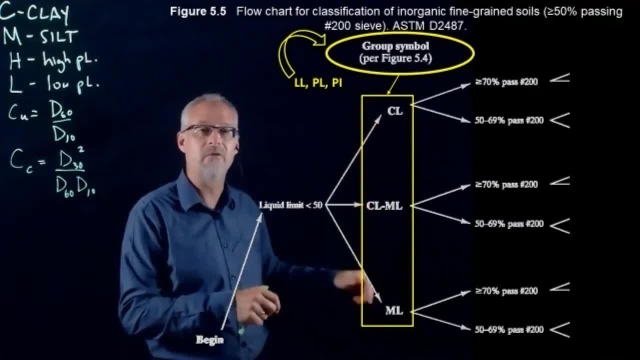 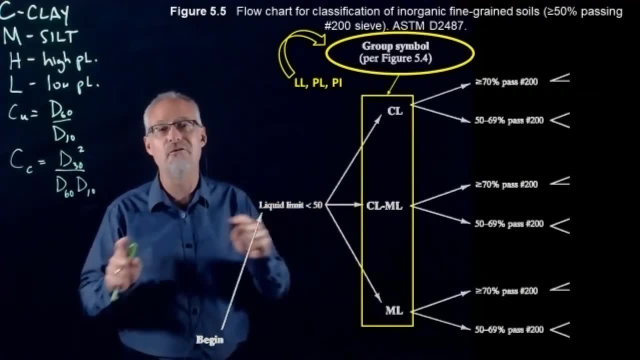 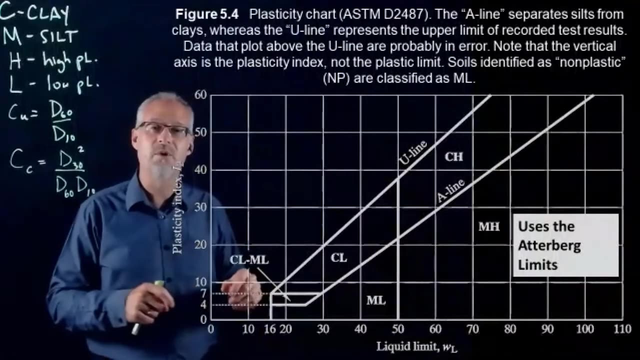 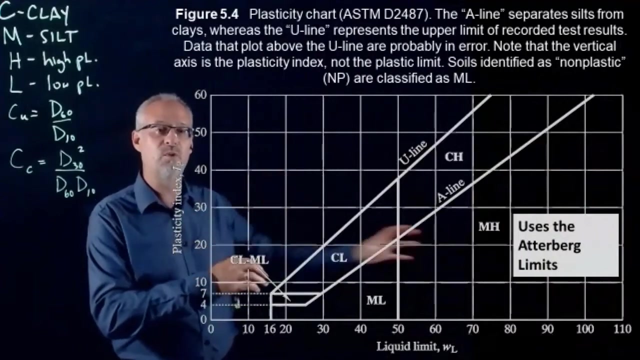 of the flow chart with our liquid limit less than 50. the next thing we do is we have to identify that two letter code. right, and that two letter code And the group symbol is coming from that chart that I talked about before this one. Okay, so we're in the classification process and we reach the decision point of: okay, where does it fall on this figure? 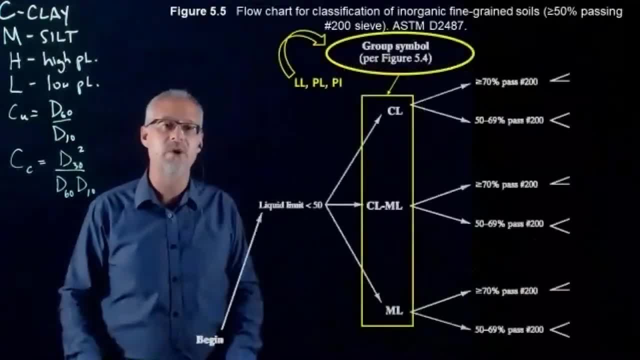 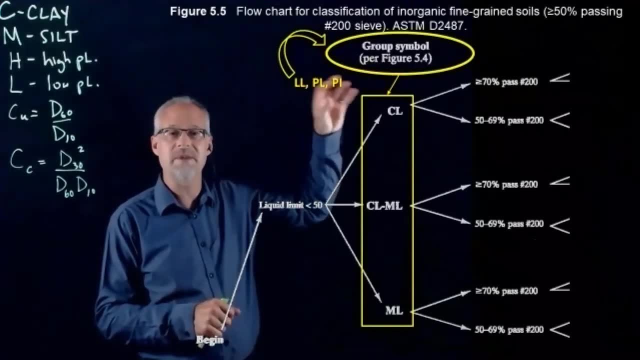 We call it figure 5.4 in this particular text. So we get to this figure 5.4, and the data is coming from the liquid limit, plastic limit and plasticity index, which is just liquid limit minus plastic limit. 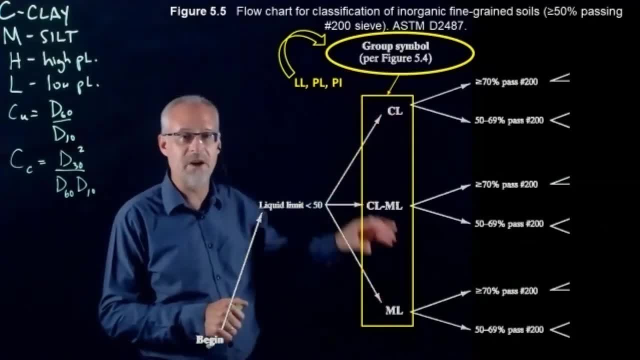 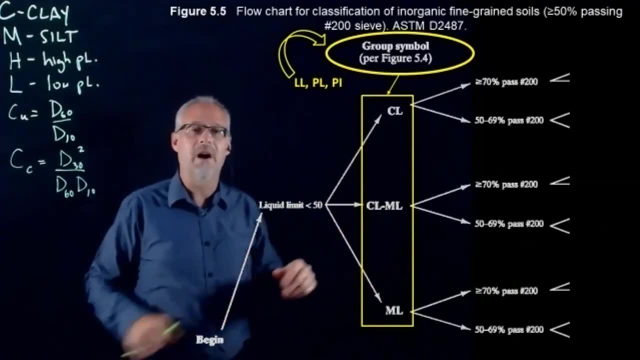 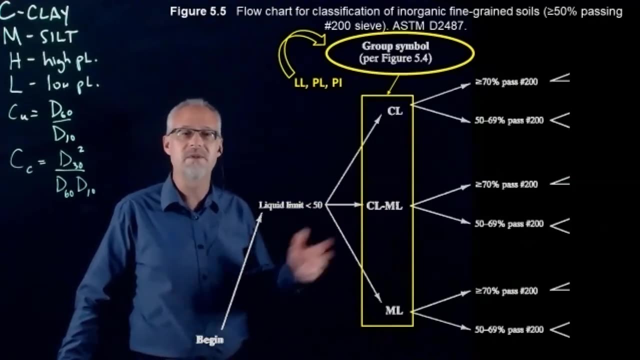 So then we give it either a CL, a CL slash ML, or an ML, And notice that I'm not going to get an H in here anyway, because my liquid limit is less than 50. So if I have a liquid limit less than 50, and my soil plots in a quadrant that's not one of these quadrants, then I've done something wrong. 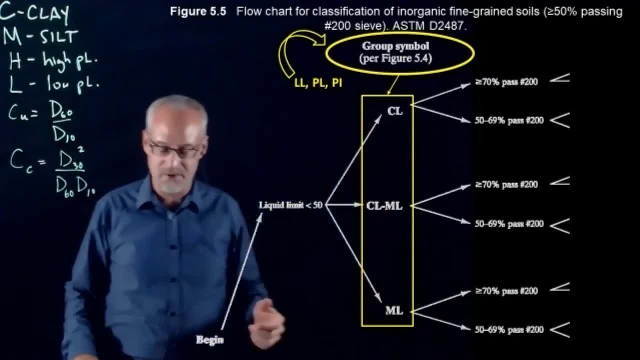 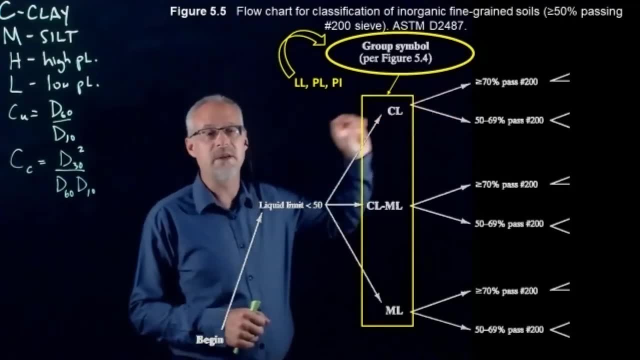 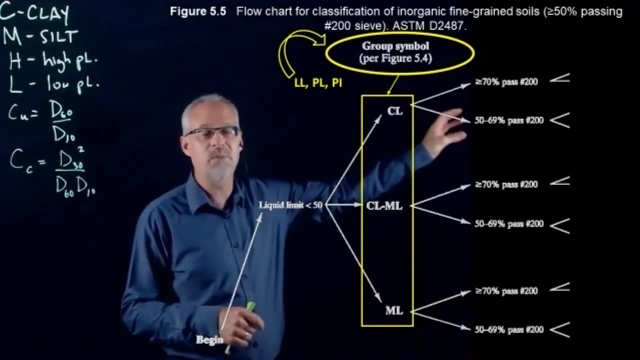 Okay, so that's the first step. The next step, depending on which one of these we fall into, we then go over and say: is it greater than 70% silt and clay, or is it between 50% and 69%? 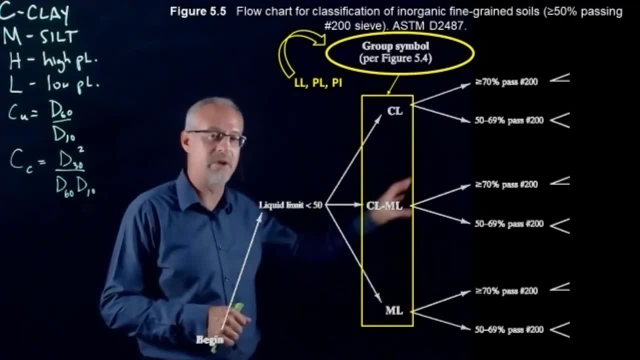 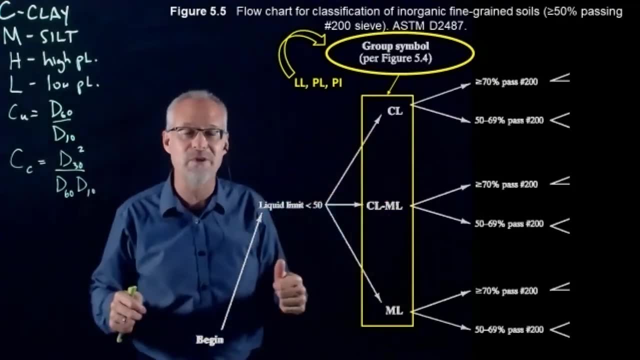 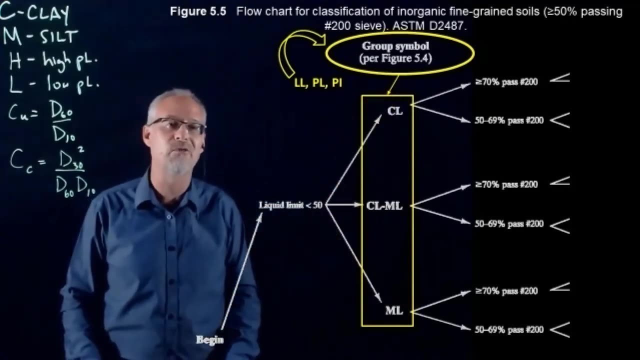 Same decision for each of these other ones. Notice that the lower limit is 50%, not zero, because in order to be using this chart, it has to be greater than 50%. Okay, so pretty logical sort of how you find your way through this, I hope, anyway, so far. 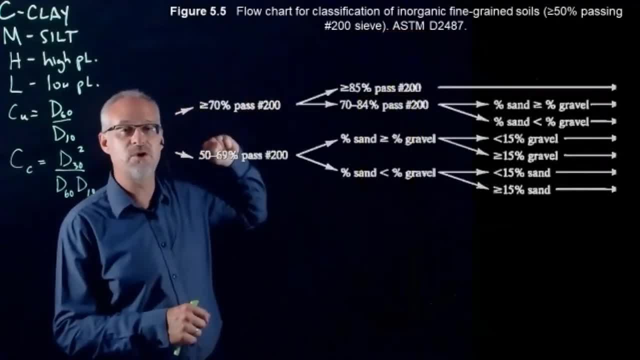 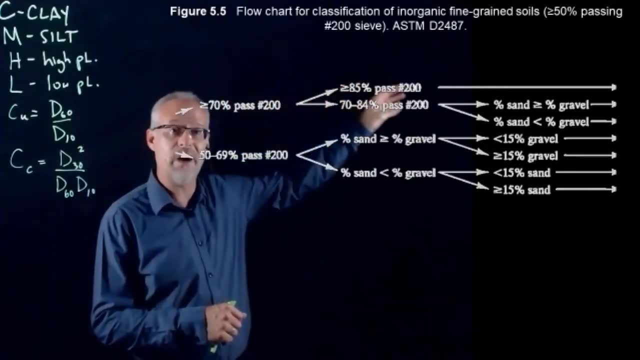 And then let's say we come to this decision tree where we go, let's say it's greater than 70% passing the number 200. Then we ask another question: is it greater than 85% passing the number 200?? Okay, 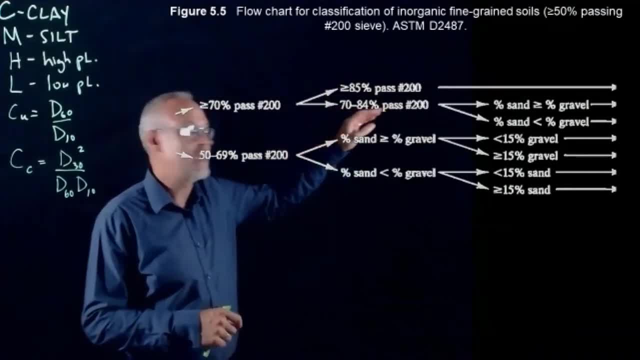 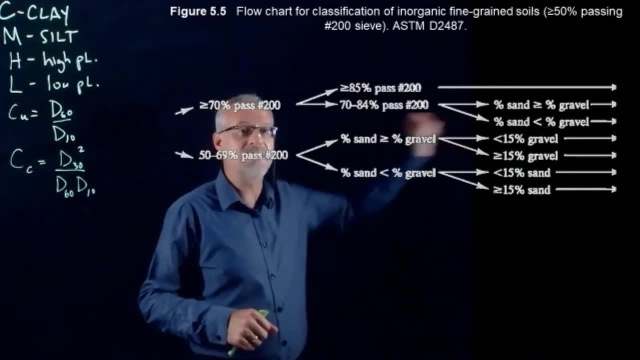 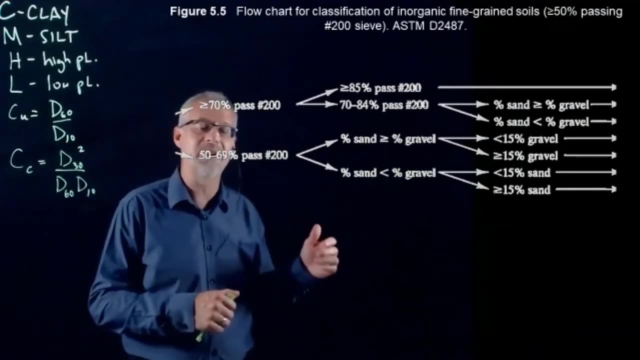 Or is it between 70% and 84%? And then, if it is between 70% and 84%, we have another decision to make, And that is: is the percentage sand greater than or equal to the percentage gravel, Or is the percent sand less than the percent gravel? 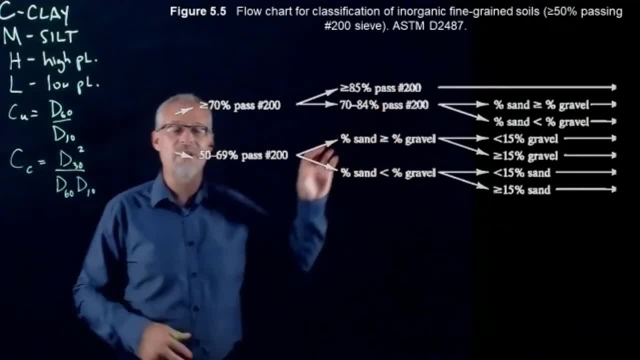 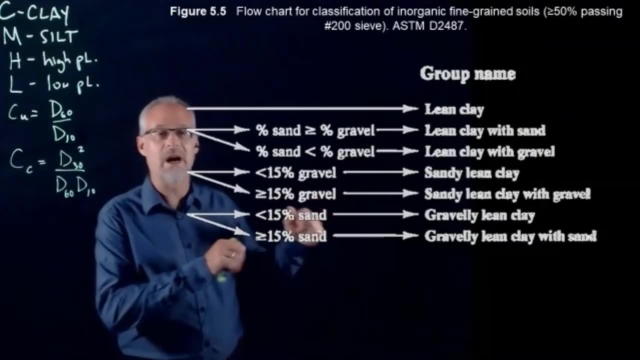 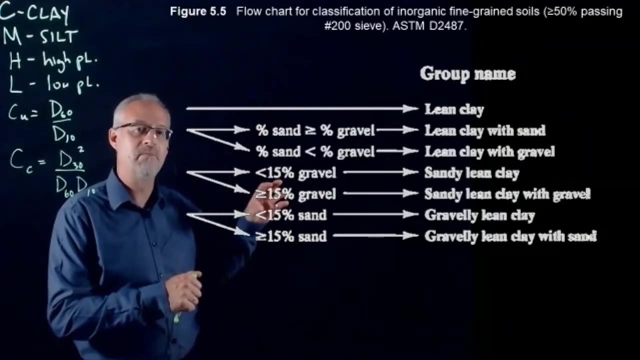 Okay, and so you need to follow these greater than or equal to sort of flow charts. pretty easy really. And then the last part of the graph, After you've identified what percent sand versus gravel, or specifically a percentage of sand or gravel. 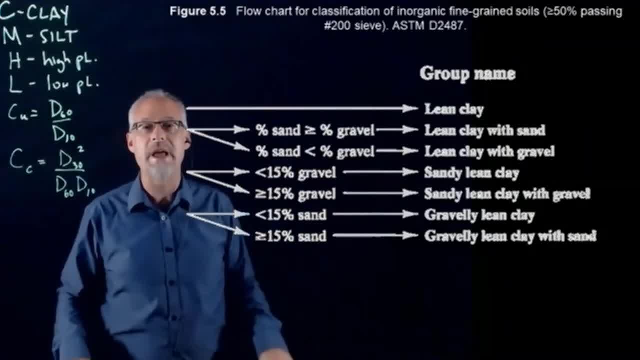 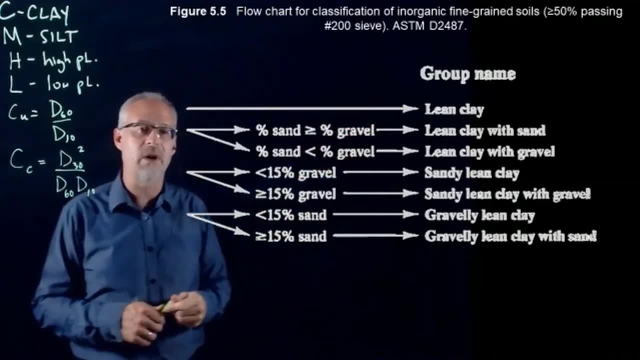 we can then actually assign the so-called group name, But you can see some of the names that we end up with. You know we can end up with a lean clay, a lean clay with sand, lean clay with gravel, sandy lean clay. 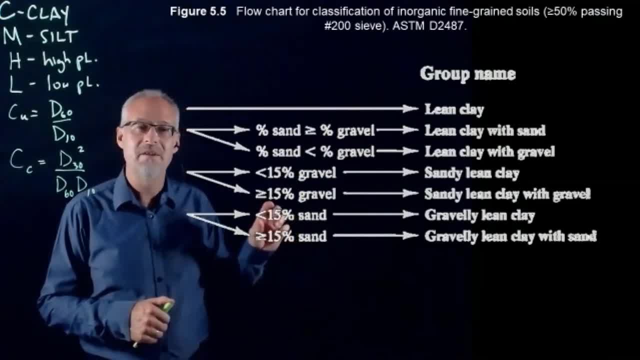 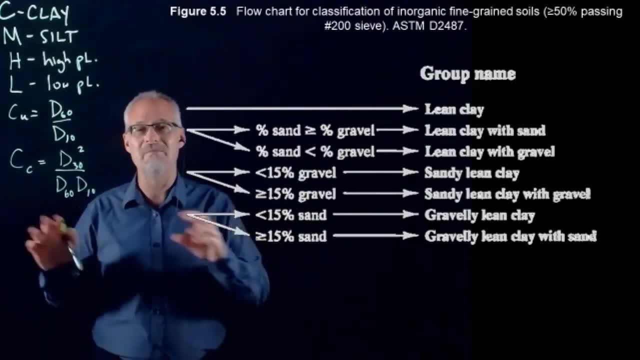 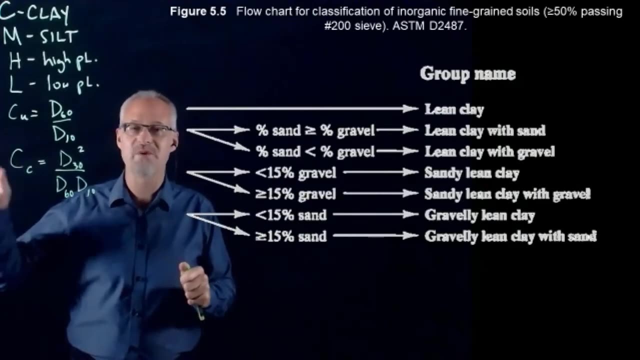 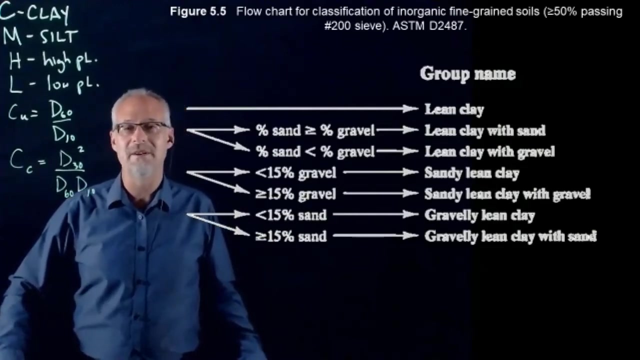 But notice that the noun is always clay, So it kind of you know it should remind you of the soil descriptions that we had from before. Those soil descriptions from last week actually came from the Canadian Geotechnical Manual, primarily used for sort of a quicker classification. 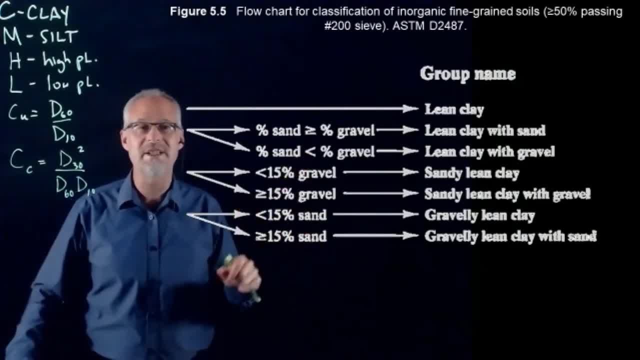 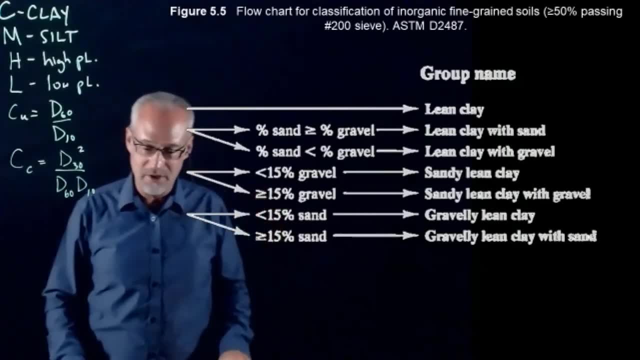 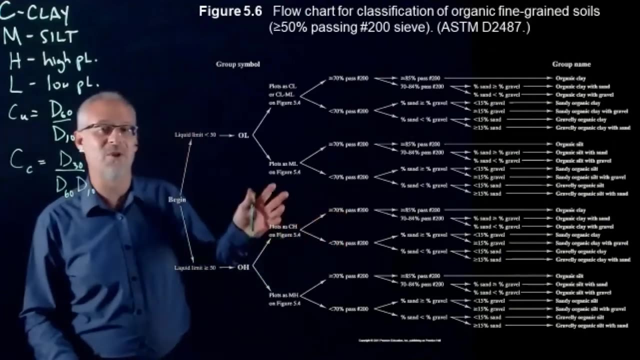 The Unified Soil Classification System has a little bit more detail to the actual so-called official group name, And it's good for you To do this. This is another flow chart that I want you to ignore And you might say: well, that's good. 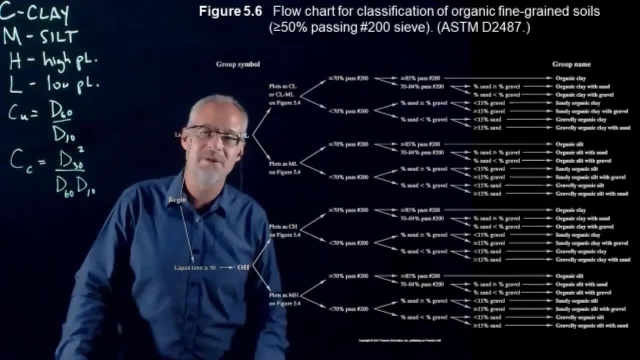 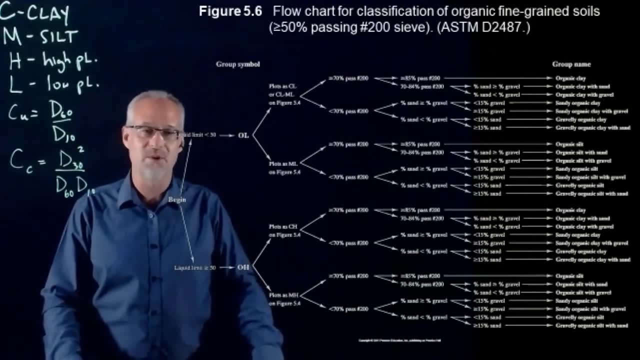 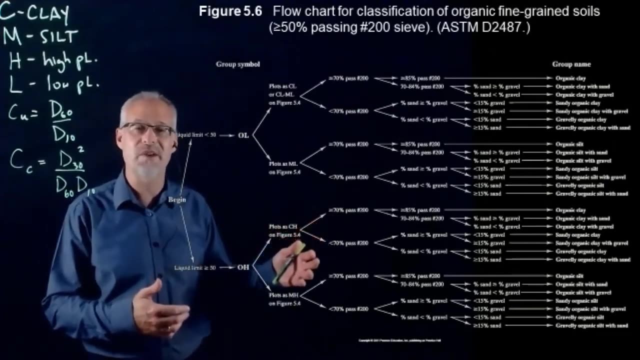 And that's because this is for organic soils And in my practice in geotechnical engineering we usually would stay away from organic soils, So they're not really something you want to build with. Just know that it's here, And the Unified Soil Classification System does deal with the classification of organics. 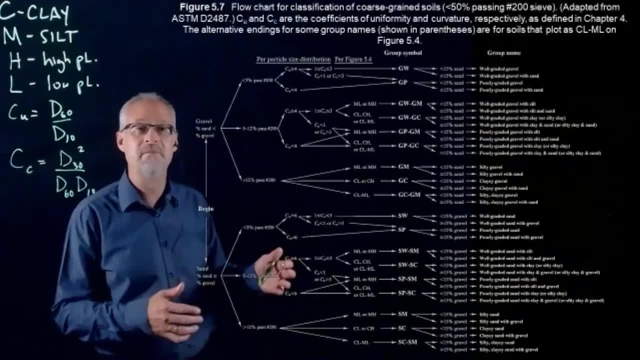 But we're not going to do that, So we're going to do this, So we're going to do this, So we're going to do this. We're not going to focus on them, But what we are going to focus on is coarse-grained soils. 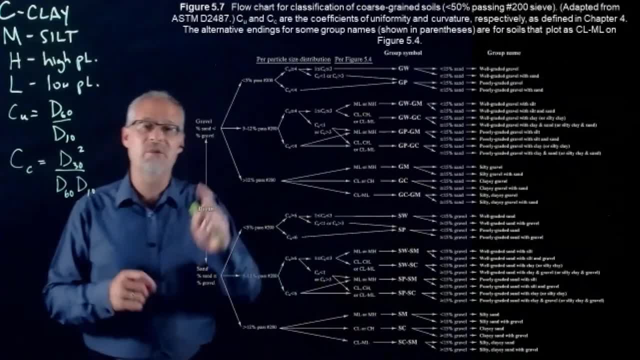 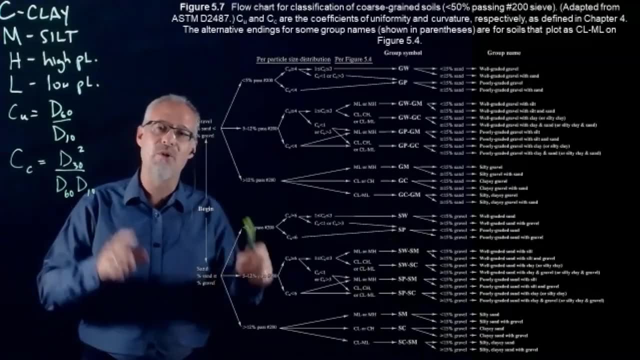 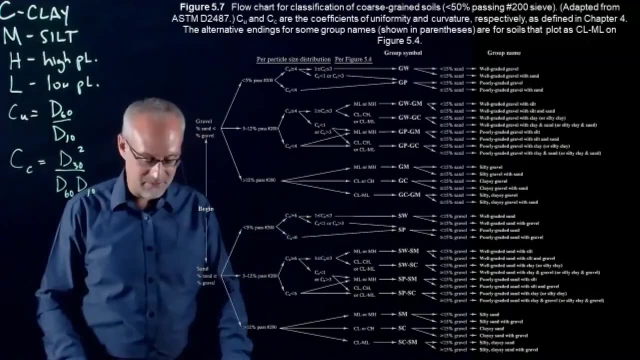 And again, I know you can't read this, So let's just step through how you classify a coarse-grained soil, And that would be a soil that has greater than 50% larger than the number 200 sieve. So it's the reverse from the first fine-grained example. 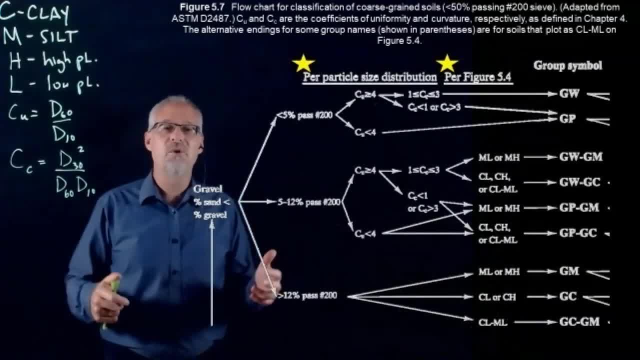 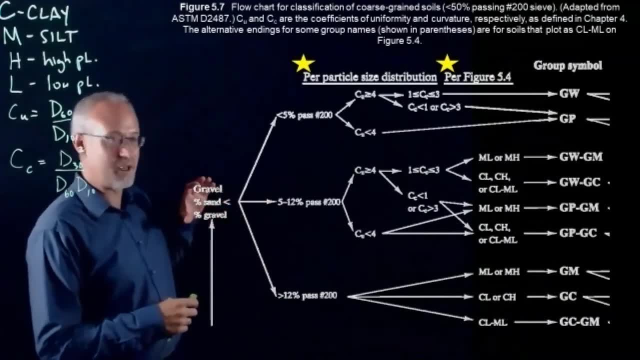 A couple of things to note. The first thing that we do in classifying is we're going to be using a coarse-grained soil as we decide is it gravel or is it sand, And we do that by saying: is the fraction of sand less than the fraction of gravel? 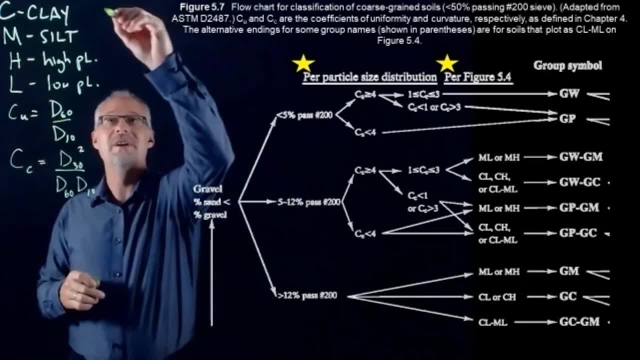 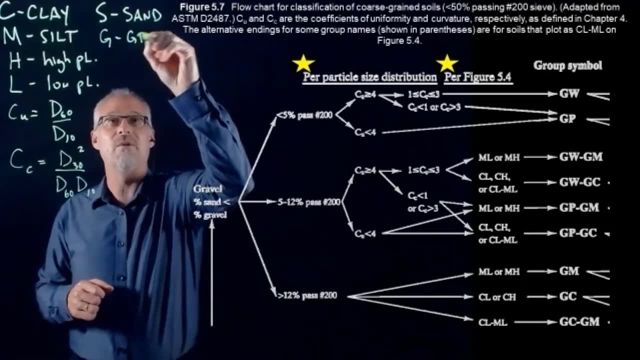 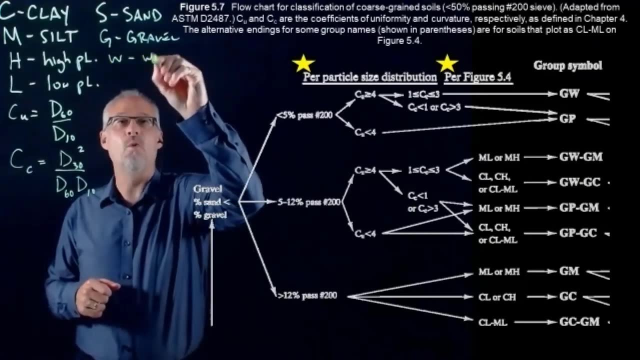 And I'll tell you what. there's a couple of other words up here. I should define the S. We're going to use S to mean sand. We're going to use G to mean gravel. We're going to use W to mean well-grained. 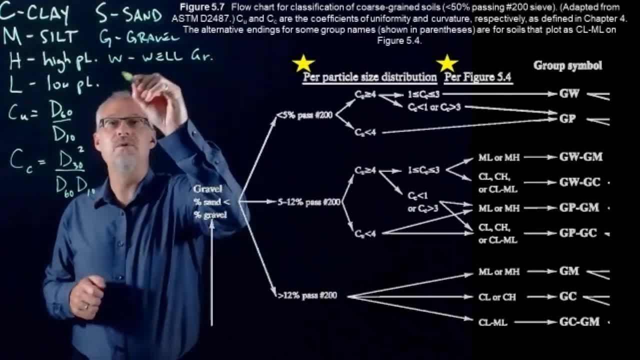 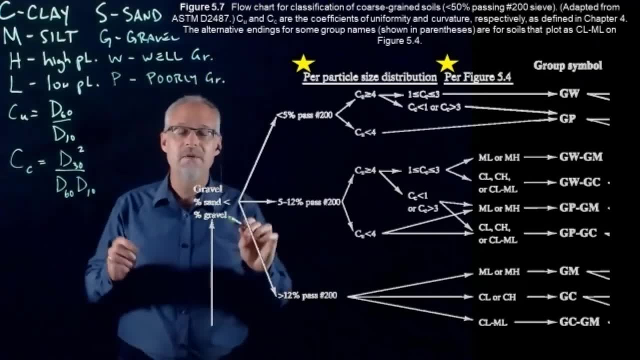 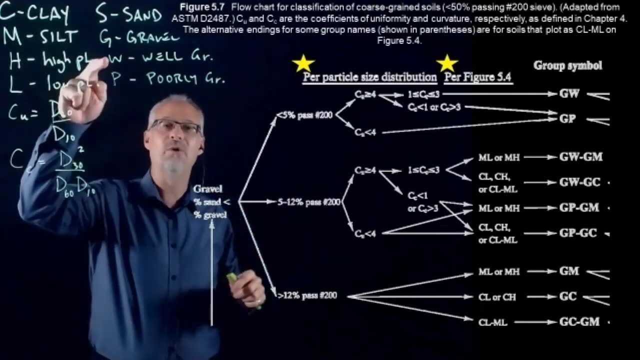 And we're going to use P to mean poorly-grained. And remember, we're going to use the geotechnical engineering meaning of the word well-grained and poorly-grained, Where well-grained means that it has a lot of different particle sizes. 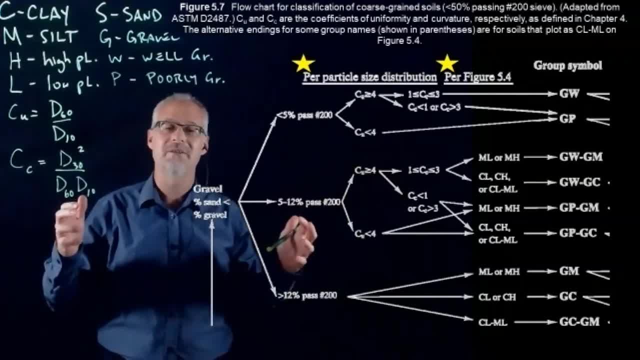 Poorly-grained means that it's kind of all one size. So poorly-grained would be like a bag of marbles. Well-grained would be like a bag of marbles. Well-grained would be like a bag of marbles. 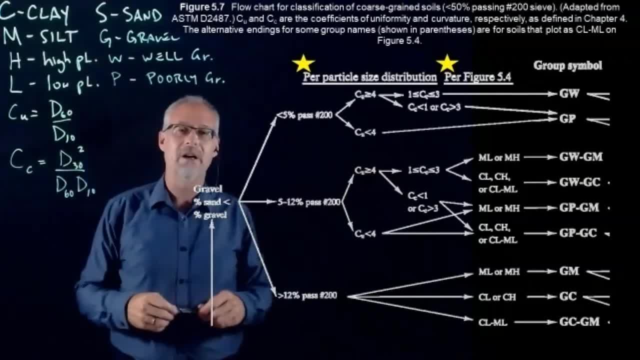 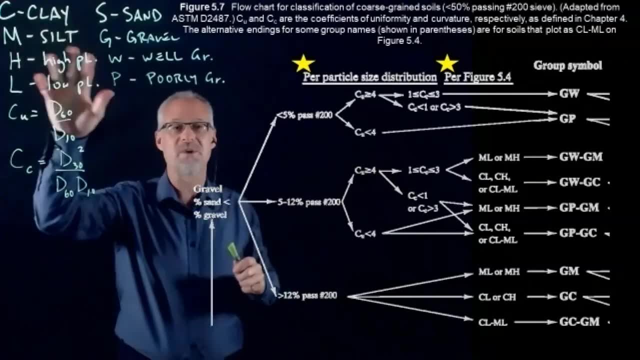 Or it could be a gravel that you want to pack very tightly, that has a wide range of particle sizes. So, again, pretty straightforward, But these are the letters that you're going to see showing up here. So, after we've determined the fraction of gravel versus the fraction of sand, 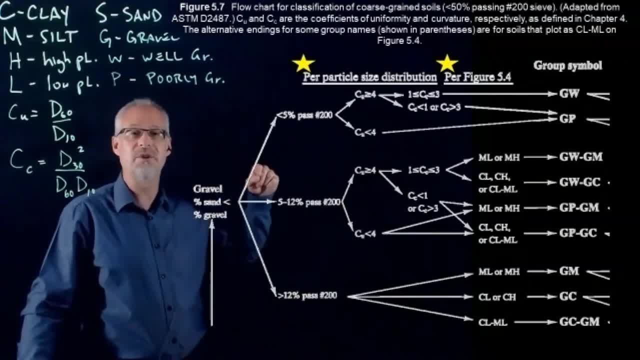 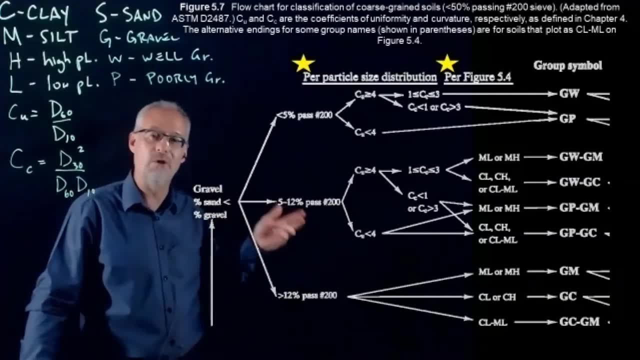 we then go down again through the grain size distribution and say, well, is it less than 5% fine grain soil, or is it between 5% and 12% fine grain soil- that's what the number 200 means- or is it greater than 12 fine grain soil? and then, depending on what, 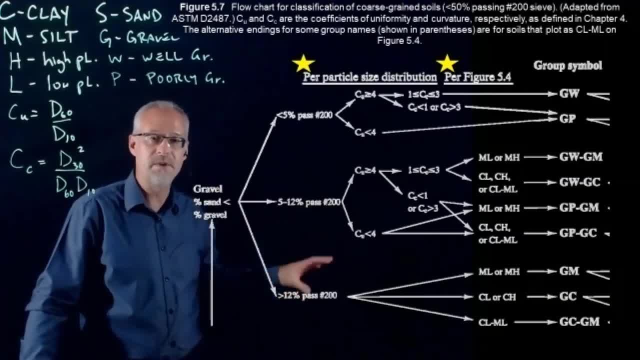 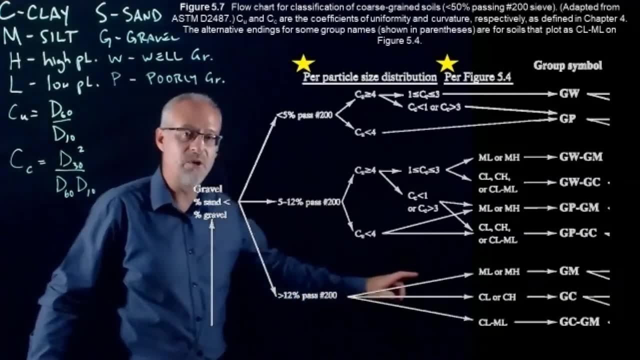 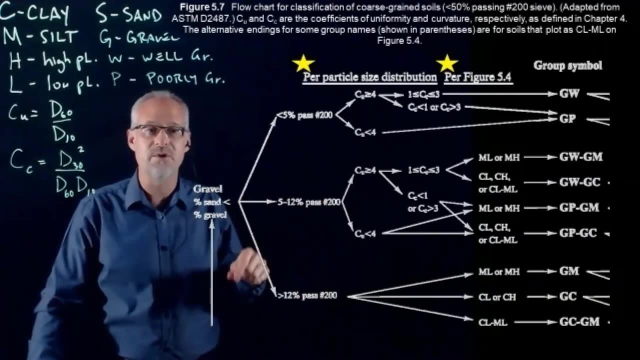 it says: so notice down here. well, for both of these there's a significant portion of fine grain soil. so so down here you'll actually have to. you'll still have to classify the fine grain soil as an ml or mh or ch or cl or cl, sort of like you did for classifying fine grain soil, which means 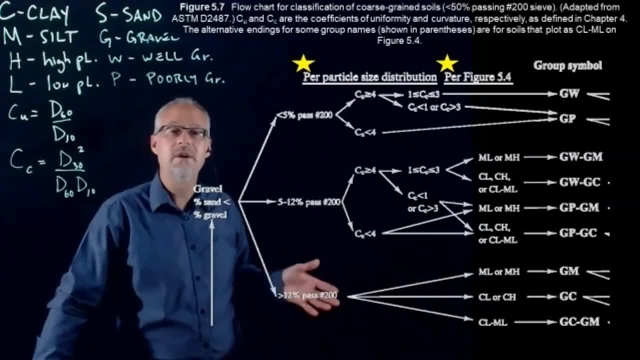 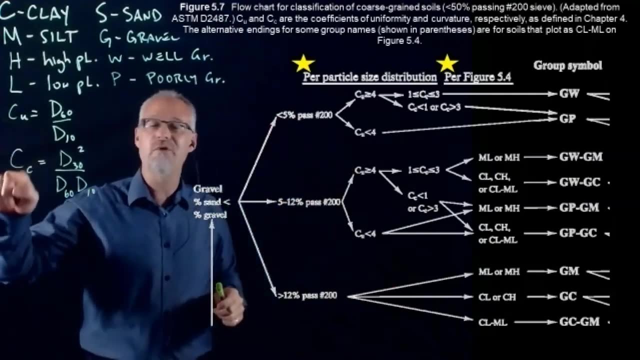 you need to run an Atterberg limits test on the percent that passed the number 200 right. so in the lab test you would need to actually do that if for these two divisions we actually have to calculate the coefficient of uniformity and the coefficient of curvature, because that's 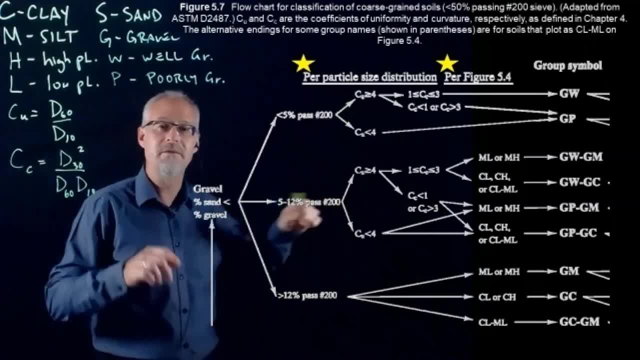 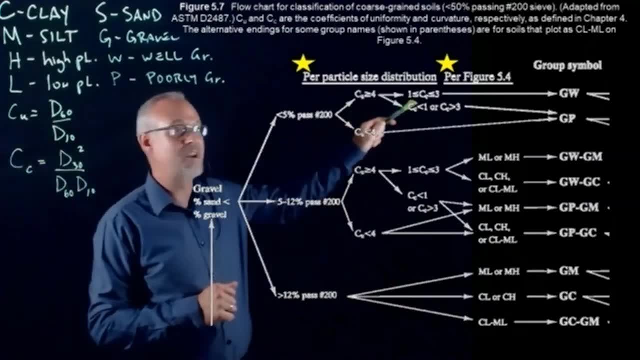 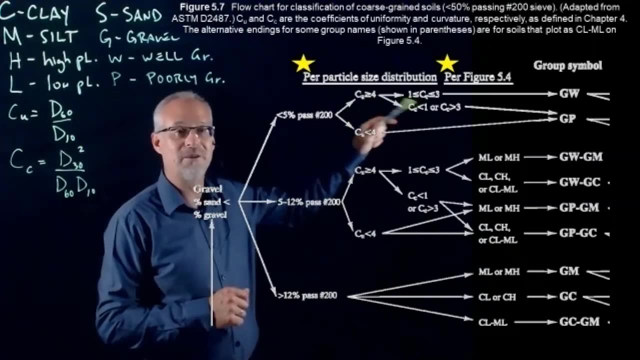 our next dividing line here in the flow chart. okay, so, so you have to be able to calculate those numbers, to follow along. and then here there's even a second check. you know, we have to do the, the coefficient of uniformity, and then we have to do the coefficient of curvature. and same thing here: coefficient uniformity, coefficient curvature. 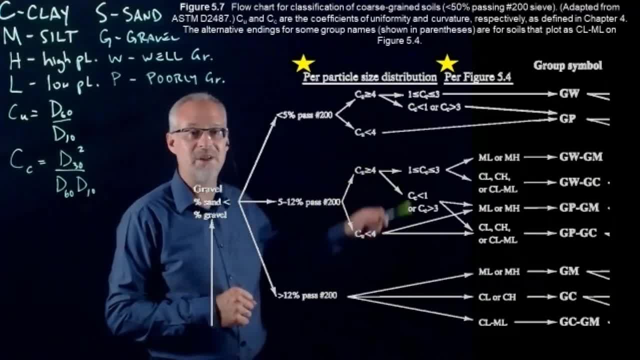 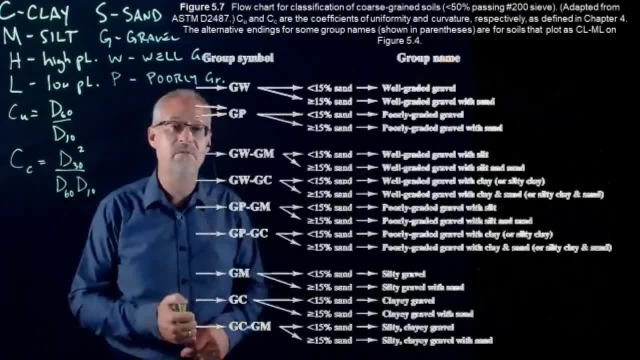 down here. we just need the uniformity, we don't need the other one, and there is even a little zone here where they cross over. okay, and then the last sort of part I zoomed in on is just where it gives you the, the group symbol, the two-letter code and the group name. 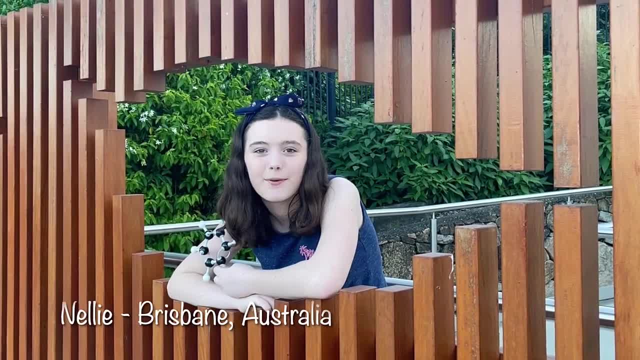 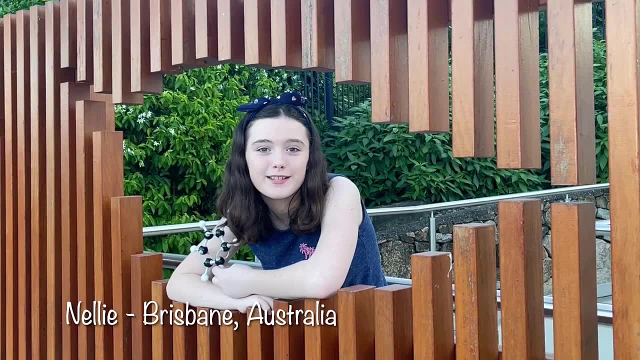 So what is the value of the biochemistry and physics literacy program, I hear you ask? Well, it teaches young people like me about how science underpins everything from medicine to the environment and even space. My name is Nellie and I am from Australia, and I get to learn all of this. 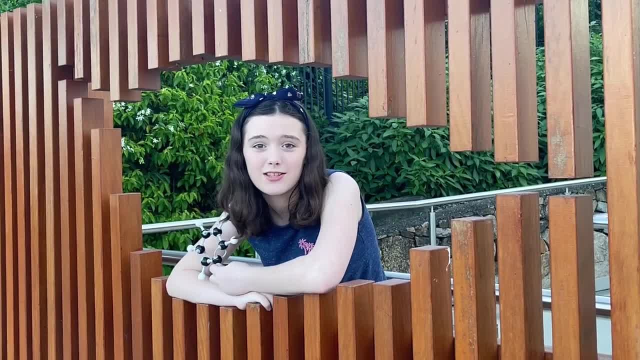 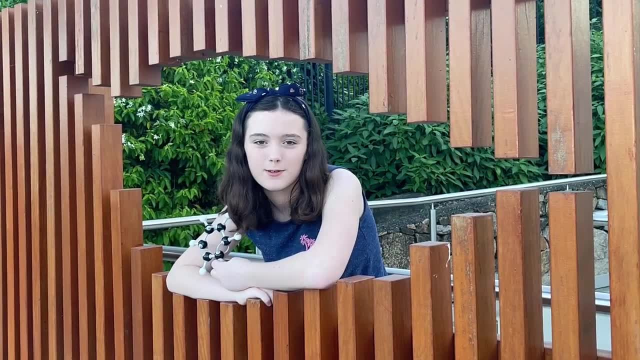 and more in a global community, collaborating and connecting with other students from all around the world, demonstrating just how globally relevant science is. One of my favorite things a part of science are the principles of neuroplasticity, which basically help you understand how you learn. 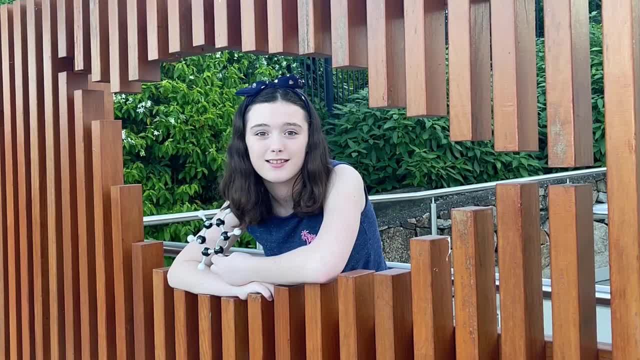 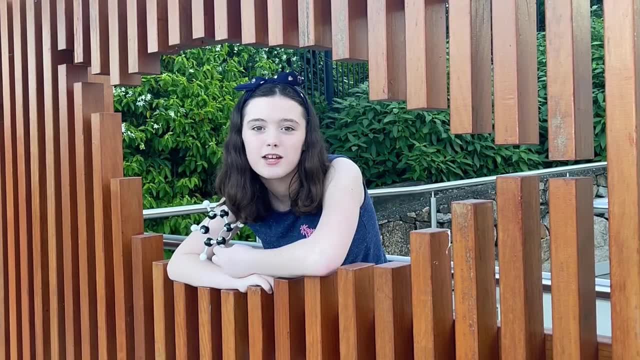 and important rule that they follow is that the younger you are, the easier it is. Having this opportunity now, at a younger age, is perfect from a neuroplastic point of view. I know that the science literacy gained will be used for other future scientific ventures. 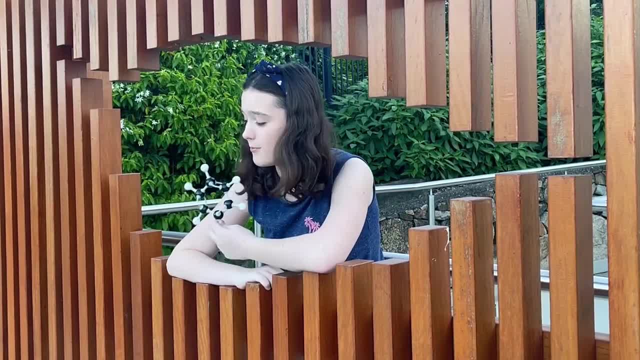 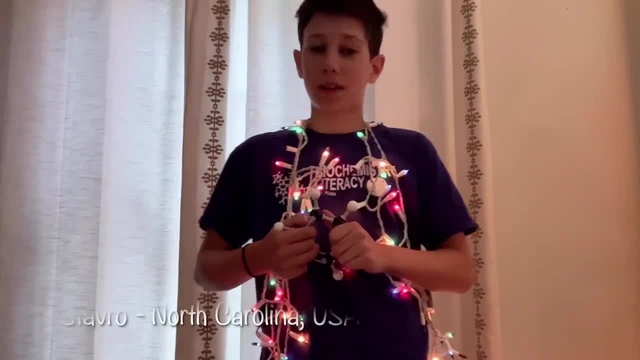 Thank you and please help support us in putting on this camp. Now I'm going to pass this here: Benzene ring to all of my friendly global classmates. Another topic we have learned about in our biochemistry class is how different colored lights work. Colored pigments are coated on the